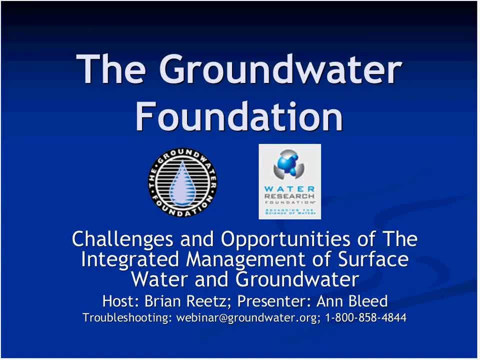 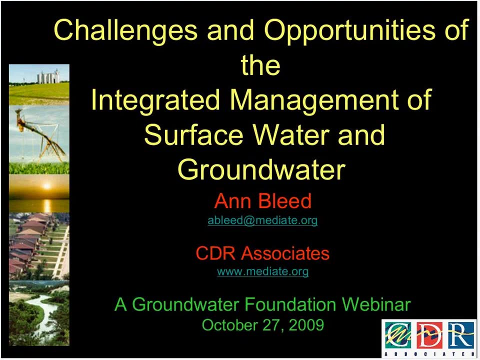 Thank you, I'll see that. As you see, it's in that box. just to the left of the send button is where you would type your question in to me. With that, I want to bring in Ann Bleed. Ann is a senior program manager with CDR Associates. 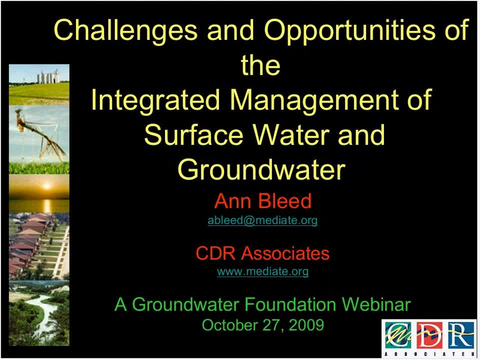 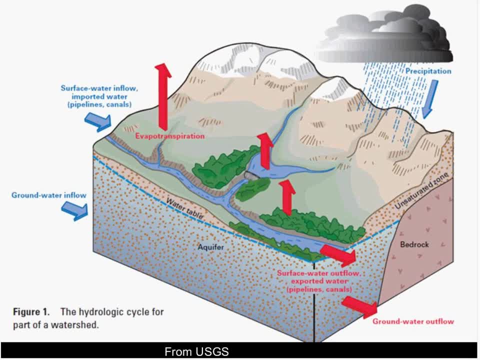 or totally consume it. As you probably all know or are very familiar with the hydrologic cycle, In the cycle we do talk about water consumption, which is primarily equated with evaporation or evapotranspiration, But these processes do not destroy water. 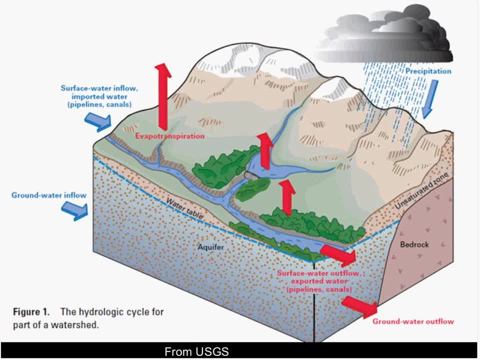 They simply remove it from the local area of interest and provide it as precipitation in some other area. Thus, our major problem is not that there isn't enough water in the world, but that the water we have is not at the right place at the right time. 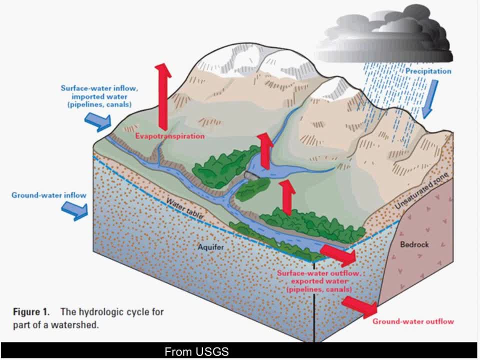 This has and already will continue to provide an opportunity, however, because it is possible to relocate and retime our water supply for more efficient, beneficial use. Pollution of our water supplies also makes them unusable, However, even though we may pollute our water supply, 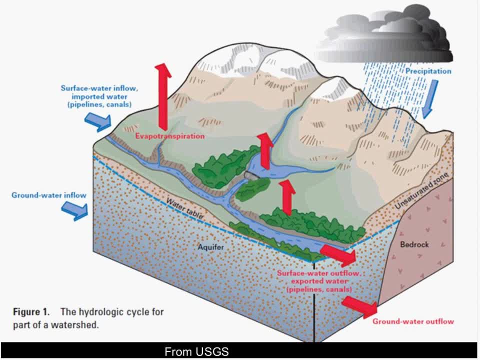 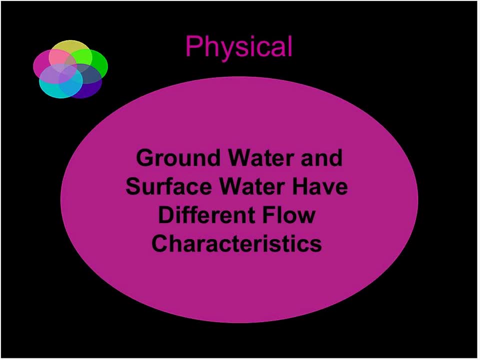 we do not destroy the water molecules in the process. Thus, we still have an opportunity. Another aspect of water that I think it's important to recognize is that surface water and groundwater have very different flow characteristics. Surface water is easy to see. We can also readily understand the impacts of our management of surface water. 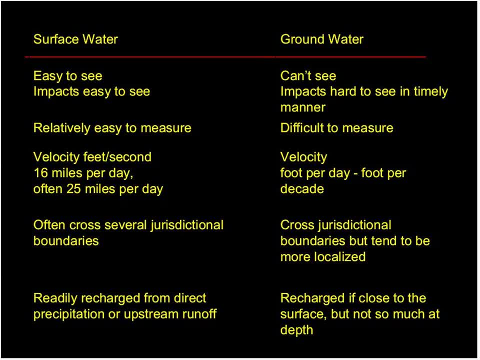 The river above a diversion dam is full of water, but below the dam it is often dry. Groundwater, on the other hand, cannot be used as a source of water, but it can be used as a source of water, So it's important to recognize that. 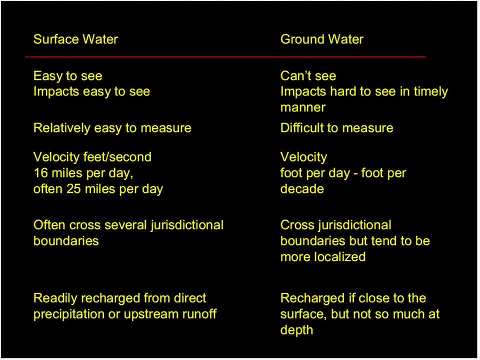 Surface water cannot be seen, is difficult to measure and the impacts of use may not be evident for many years. Surface water flows quickly- 16 to 25 miles a day- while groundwater flows very slowly, perhaps just a foot a day, or even a foot a decade. 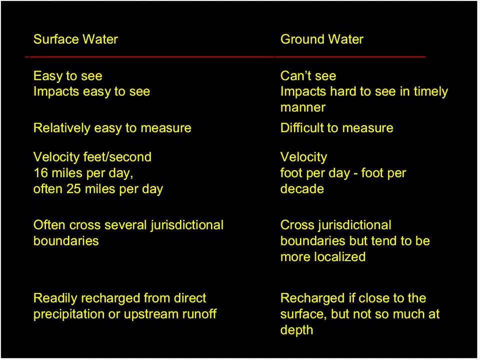 Surface water often flows across jurisdictional boundaries. Groundwater tends to be more localized. Surface water is easily recharged by precipitation and overland runoff. Groundwater, on the other hand, especially when it is in a deep aquifer, is not so easily recharged. 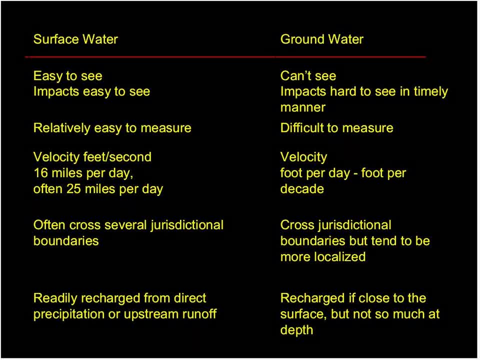 These differences in flow characteristics between groundwater and surface water create both challenges but also opportunities. For example, because groundwater flows slowly, we can use groundwater aquifers, not surface water reservoirs, which inundate land and have high evaporation rates, to store water. 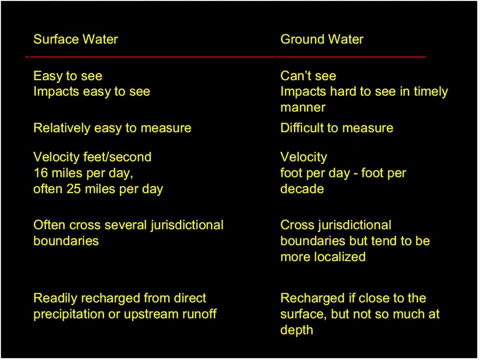 And where surface water has been diverted. aquifers have often been recharged, usually accidentally and incidental to the surface water use. However, we have learned from the results of this incidental recharge that it is possible to manage these systems, and by intentionally managing the systems. 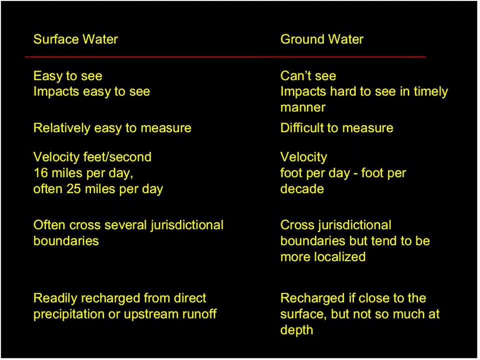 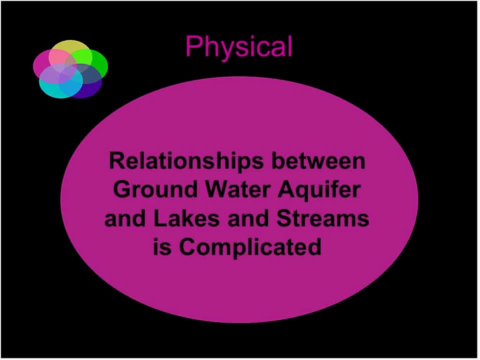 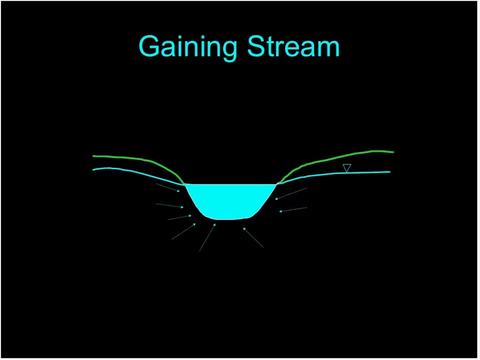 we are starting to make more efficient conjunctive management of the entire system. Relationships between surface water and groundwater- Surface water and groundwater, however- can be quite complex, and this creates a number of both challenges and opportunities. I am sure you are all familiar with the relationship between an aquifer and a gaining stream. 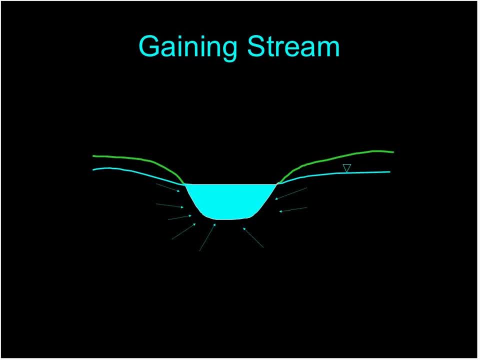 Here you see the land surface in green, the water table surface in blue and this would be the stream. This would be a gaining stream where water is flowing, The water is flowing from the aquifer to the stream, as opposed to a losing stream, where water flows from the stream to the aquifer. 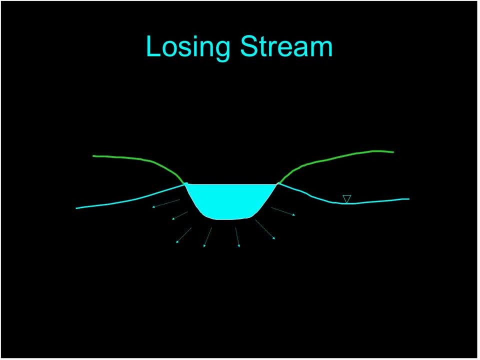 The relationship between a gaining stream and a losing stream is very definitely a dynamic system and the relationship can change quickly depending on weather conditions and weather use, even within one day, As mentioned previously. the impacts from groundwater pumping, on the other hand, may take a long time to be recognized and to see. 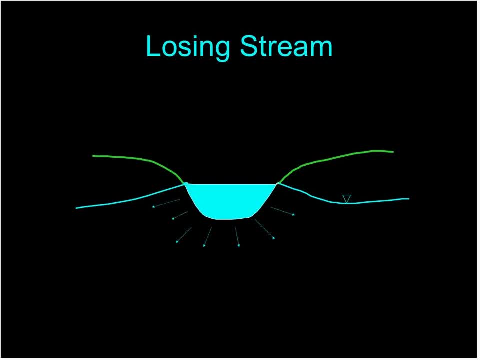 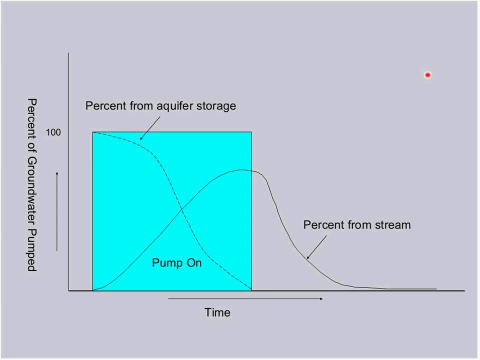 in part because of the complex relationships between surface water and groundwater. Let me explain a little bit further. This is a chart showing the impact of a pumping well on a stream and the source of water for the impact of the well. On the vertical axis you see the percent of water that is going to the well that is pumped. 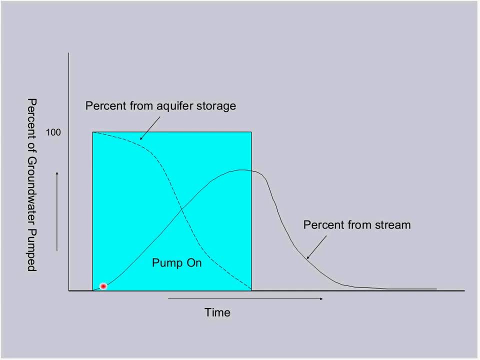 and in the horizontal axis is time. The blue rectangle indicates the time at which a pump is turned on and is pumping water At first. when the pump is turned on, about 100% of the water in the storage in the aquifer will go to the pump. 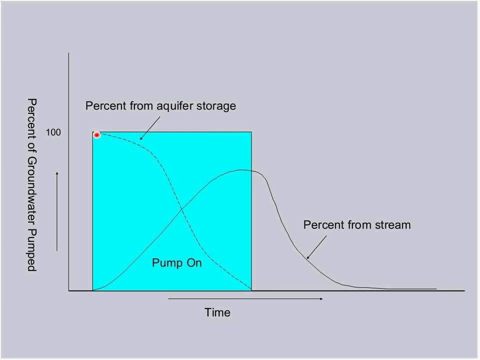 and all the water from the pump will be coming from the aquifer. As time goes on, however, the amount of water coming into the pump will start coming from the stream, and this will increase over time. Now, the water that is going into the pump is not necessarily being sucked from the stream. 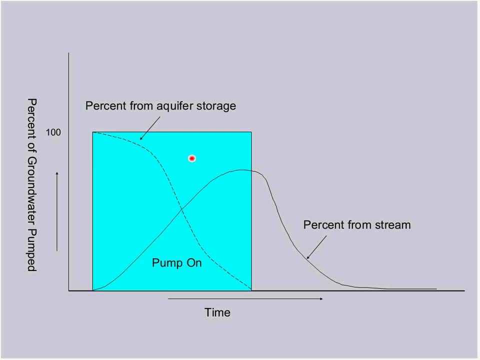 but the pump is intercepting water that otherwise would go to the stream. Once the pump is turned off- indicated here- the impact of the pumping of the well on the stream will continue for some time. The length of time that the well will impact the stream. 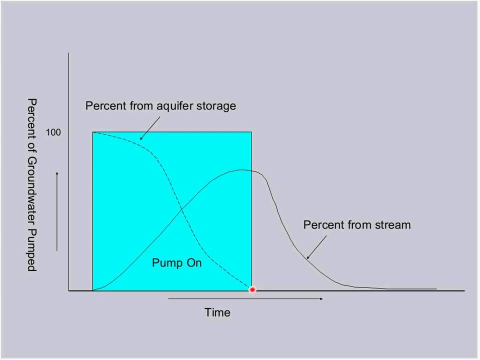 depends on a number of physical characteristics. A well close to a stream will have a fairly fast impact on the stream. A well at some distance from a stream may not have a noticeable impact on the stream for years, decades or even centuries. This lagged impact of wells on streams provides opportunities. 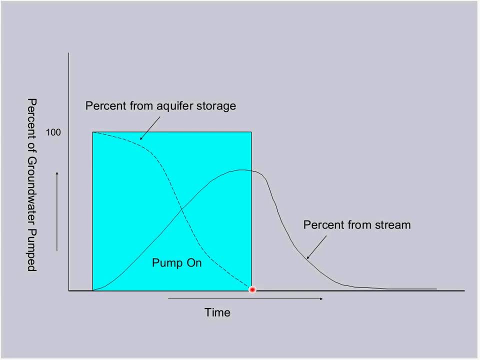 for managing the lag to provide better timing of water availability to meet our demands, but it also complicates our ability to predict the future impacts of a well. In addition, a well at some distance from a stream may not have a noticeable impact on the stream. 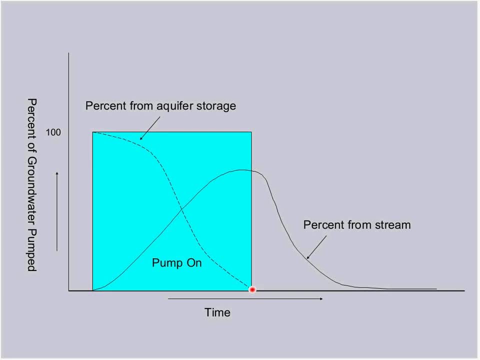 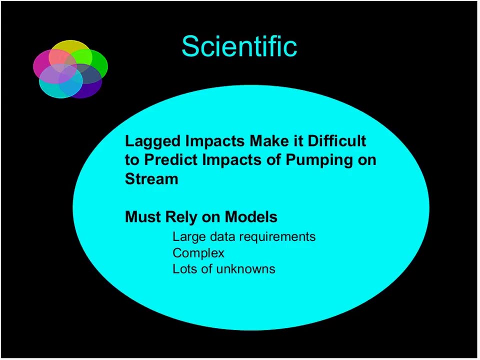 This lagged impact of wells on streams provides opportunities for managing the lag, to provide better timing of water availability to meet our demands, but it also complicates our ability to predict the future impacts of a well on a hydrologically connected stream, which leads me to my next topic. 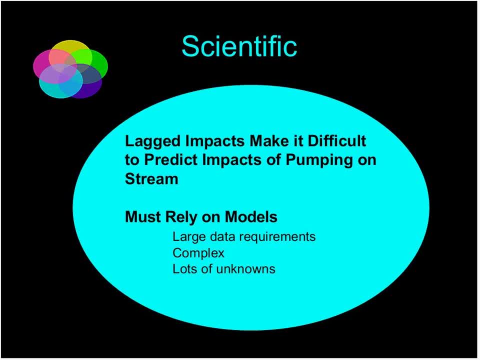 To predict the timing of impacts of a well on a stream, we must rely on complex groundwater-surface water interactive models, which usually require large amounts of data. Rarely is all the data we desire actually available. This creates tremendous scientific problems To develop an accurate model. 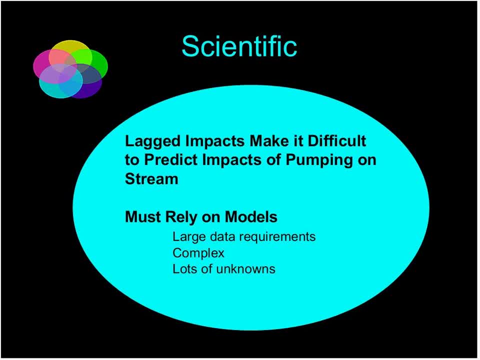 the standard practice is first to develop a model that emulates the historical conditions of the stream aquifer system, And once the model is accurately able to reproduce what happened in the past, we use it to predict what will happen under a different set of conditions. 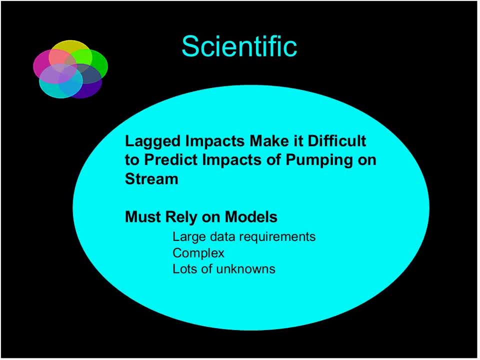 But often the records for the past are not available. For example, rarely do we have historical records on how much water was actually pumped by groundwater wells. Aquifer recharge is another critical input to models for which we rarely have actual data and therefore we mistake estimates of what we think the recharge should be. 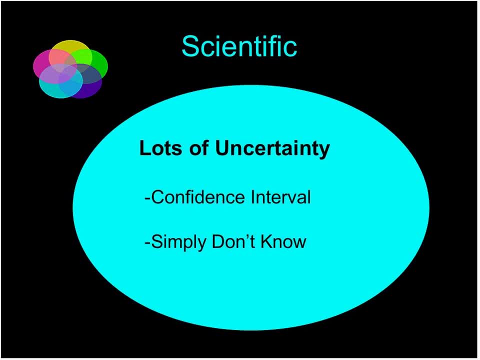 These scientific problems lead to a tremendous amount of uncertainty about the model output. Some input data. we may be able to put limits or confidence intervals around to assess the risks that the data may be wrong, But in other cases we simply do not know. 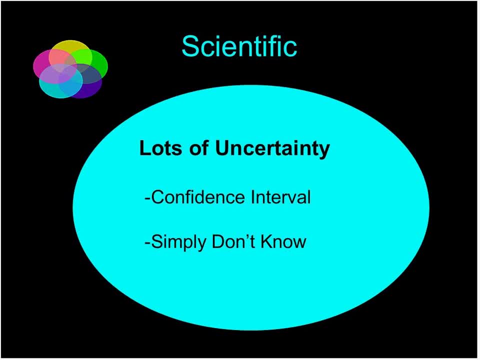 and therefore we can't even assess the risk. Yet, even though we don't have precise understanding of the basic geology we would ideally like to have, we often have to move ahead with a management decision based on the imperfect model, even when we know this decision will have major and very significant. 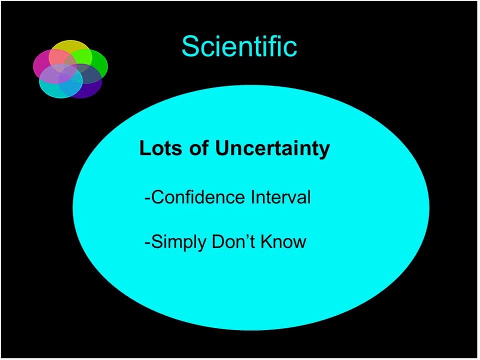 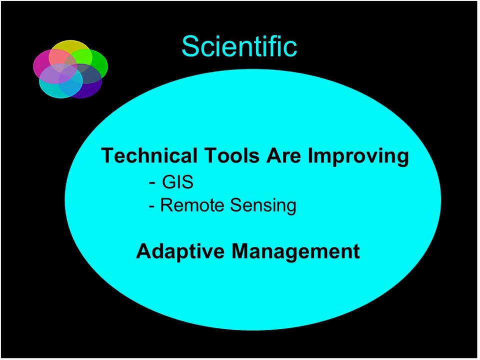 economic and environmental impacts on stakeholders. For this reason, we need, I believe, to be honest with the stakeholders about what we know and don't know and estimate the best we can what the risks and uncertainties are. On the other hand, we do have many new and developing scientific tools. 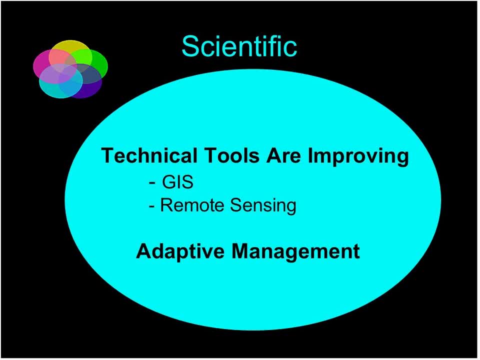 that will improve our ability to assess risk and uncertainty In particular. as an example, we have a lot of geographic information systems and remote sensing capabilities. I'd like to mention one that the University of Nebraska is working on with the help of Richard Allen from the University of Idaho. 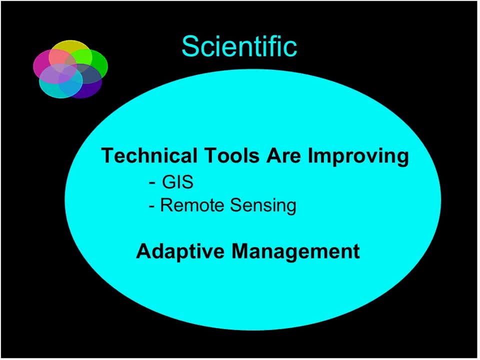 where we are using remote sensing to actually measure not just what water is being pumped, but how much water is being consumed and not returned to a local land system. It is systems like this that I think will be extremely helpful in the future. Another process that is becoming more and more important. 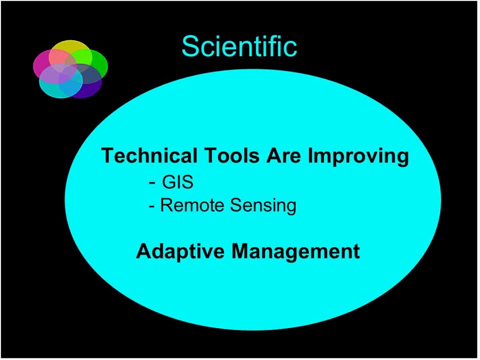 I believe, is adaptive management, which allows us to move in the face of uncertainty and be able to manage by designing our treatment processes in incremental steps so that we can test the basic hypotheses on which we are basing our management options, In addition to the fact that we are using remote sensing. 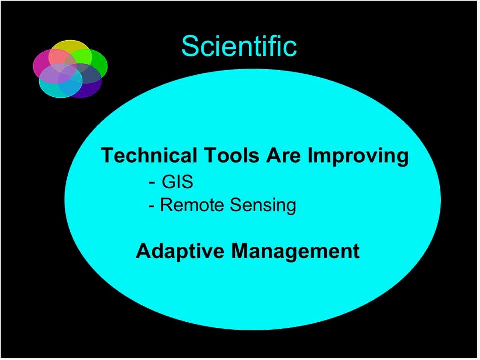 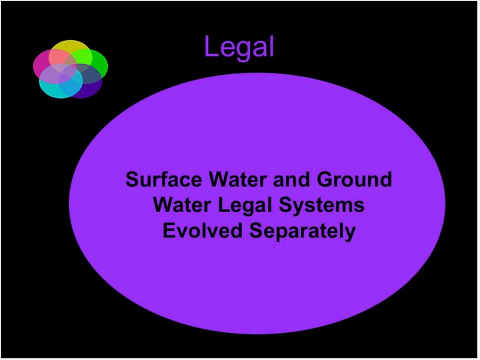 in addition to the physical and scientific challenges, there are also legal challenges In the United States. except for federal laws primarily pertaining to water quality, water law is developed and administered by the states, not the federal government. Surface water and groundwater law in the US evolves separately. 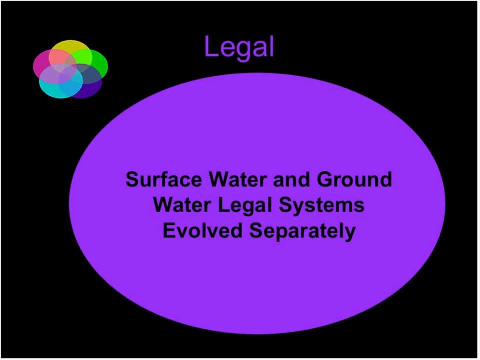 In the western US, where water tends to be scarce, surface water law has a relatively long history. In the latter half of the 19th century, western states adopted for the most part the prior appropriation system, in which the first in time to get a permit 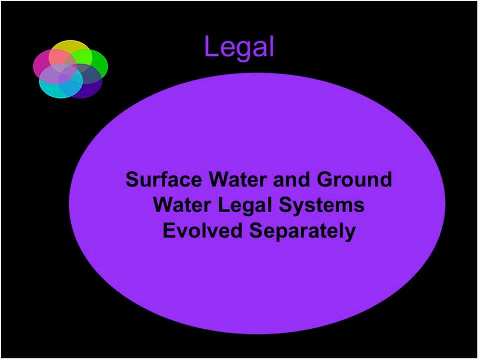 has the first right to use water. On the other hand, groundwater was rarely regulated until the second half of the 20th century. In fact, most interstate compacts and decrees, which were primarily developed in the 20s and 30s, 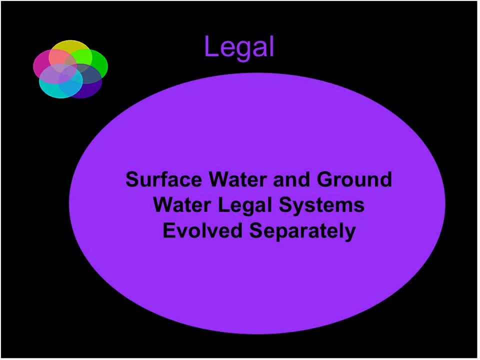 do not even mention groundwater. As a result, in recent years, there have been a number of disputes over the impacts of groundwater use on interstate apportionments. Like the interstate compacts, early groundwater law was also the result of court cases more than legislative processes. 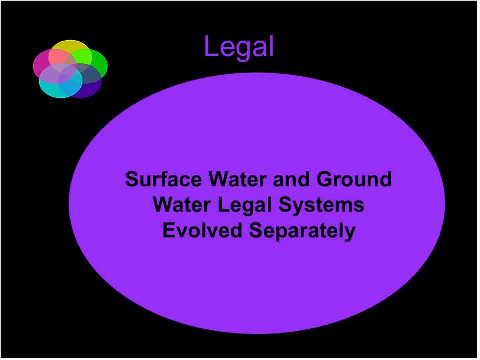 Now, however, most states have legislatively adopted the prior appropriation system for groundwater And in those states, the state itself regulates groundwater. In Nebraska, however, groundwater law is based on the concept of reasonable use, Ie you don't waste the water. 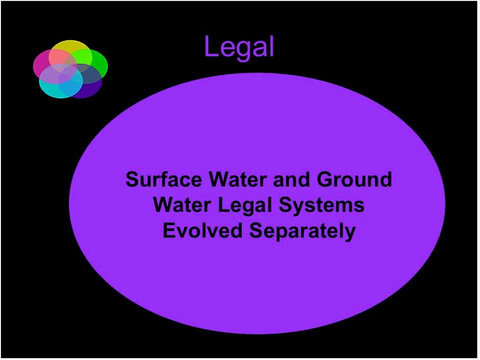 and correlative rights, meaning that in times of shortage, the water supply is shared. Nebraska also is different from most of its western neighbors in that the groundwater is not regulated by the state, but is primarily under the local control of 23 locally elected. 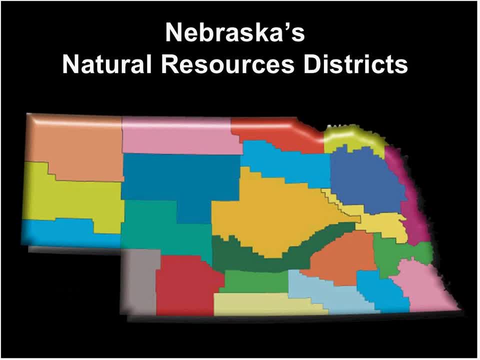 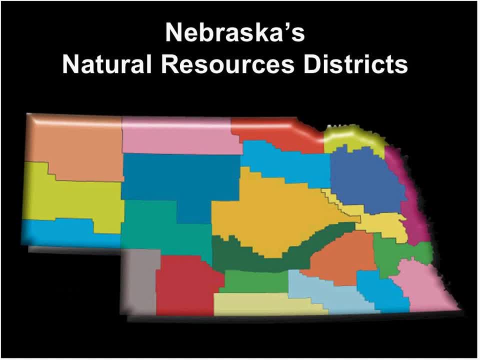 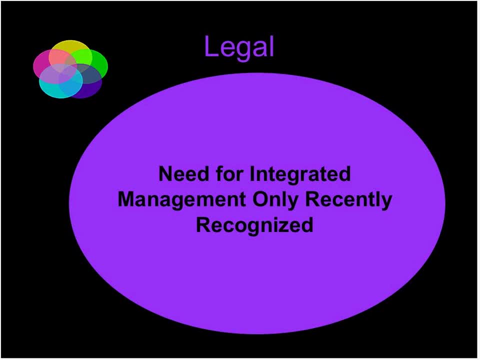 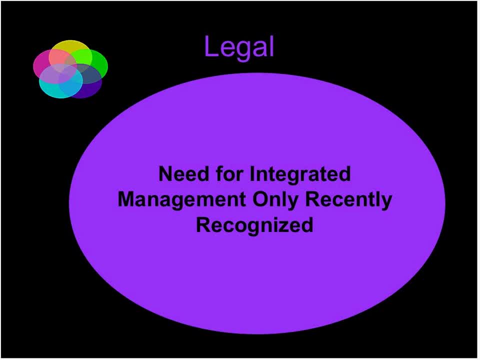 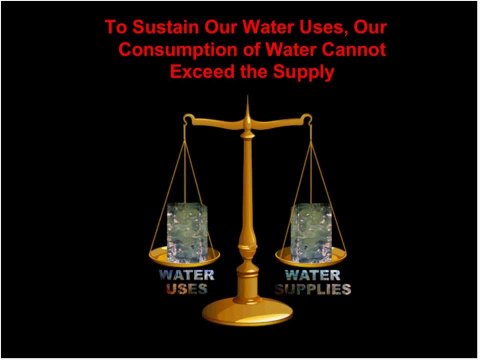 is regulated by the state itself, And I'll turn to this presentation here. I will talk about how groundwater is regulated by the state itself. That's why I uses of water cannot be sustained in the long term. The fact that this happened relates back to the complexity. 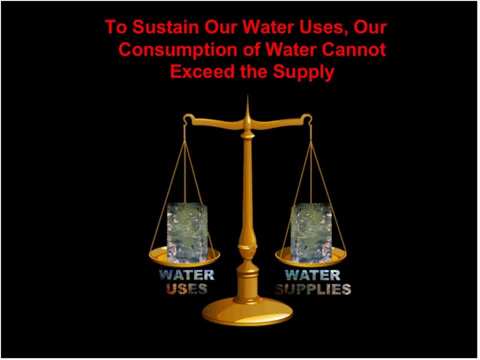 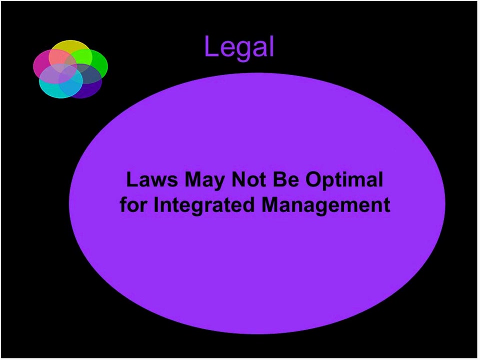 of understanding groundwater impacts and the lag effect of these impacts on surface water supplies. And even when legal systems did recognize the connection, the legal system itself was rarely adapted to accommodating an integrated management system. In most states, groundwater use was put into the priority system. 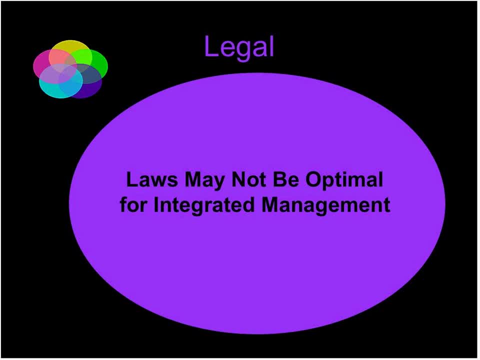 with the surface water users, So the groundwater users tended to be junior to the more senior surface water users. However, regulating a well that does not have an impact on the stream for many years is difficult to do in a first-in-time, first-in-right system. As a result, 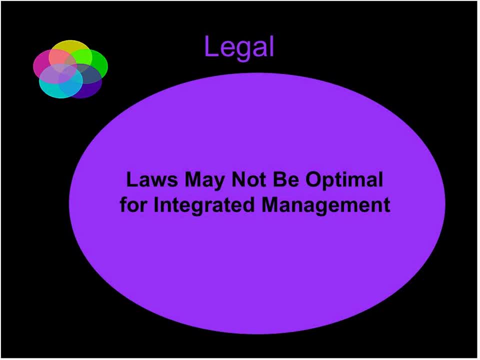 states like such as Colorado have developed a fairly complicated regulatory scheme that relies heavily on groundwater modeling and the development of often complex augmentation plans. The cost and time delays involved in developing an augmentation plan and getting the permit have resulted in a cumbersome water transfer system that has 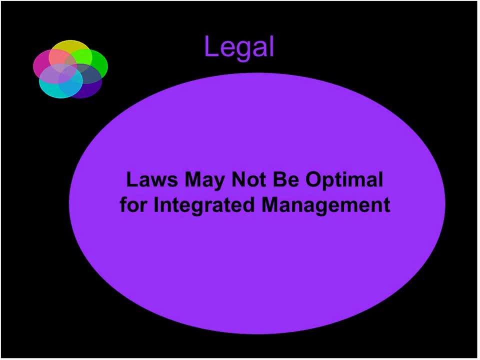 inhibited the most efficient use of water. Finally, because of separate evolution of surface water and groundwater, I think that the current laws may not be sufficient to address the current issues. I think that the current laws may not be sufficient to address the current issues. 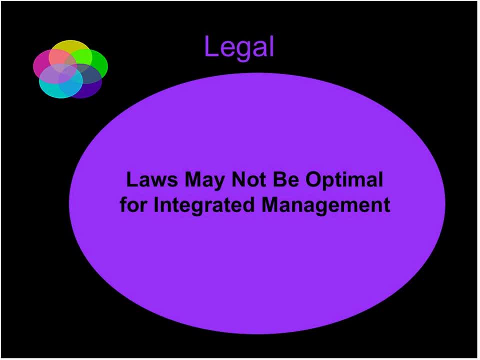 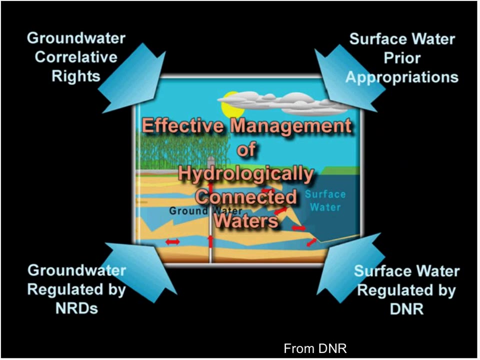 I think that the current laws may not be sufficient to address the current issues: The fact that there is some local regulation commission from the US filled with- and similar additional formulations, law that maintained a priority system under state control of the Department of Natural Resources or DNR. 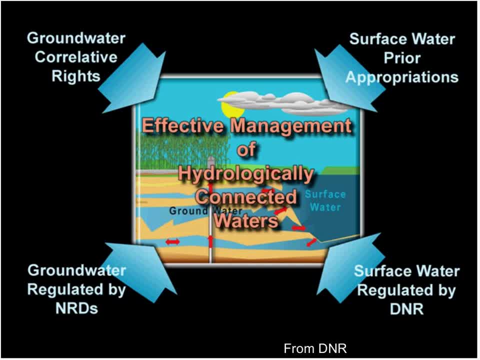 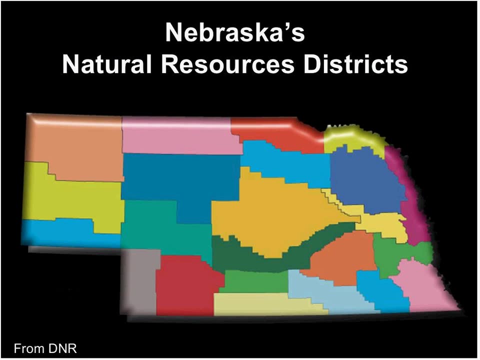 for surface water and the correlative rights system under the local control of the Natural Resources District, the NRDs, for groundwater. Under this law, the State Department of Natural Resources makes a determination of which bases are fully appropriated. This determination then triggers a three- to five-year planning period in which the state 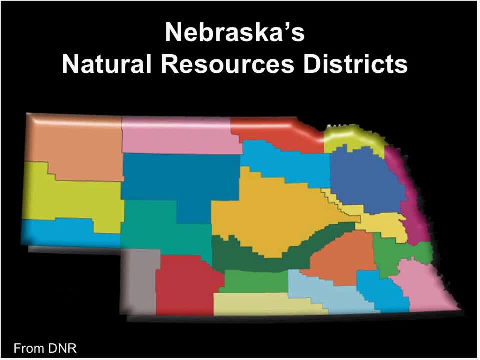 and the affected Natural Resources Districts must develop an integrated management plan for the fully appropriated basins. The plan has to have a goal of achieving and maintaining a balance between water supplies and use, so that the economic viability, social and environmental health, safety and welfare of the river basin. 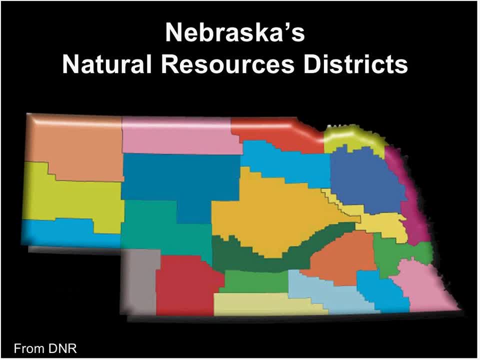 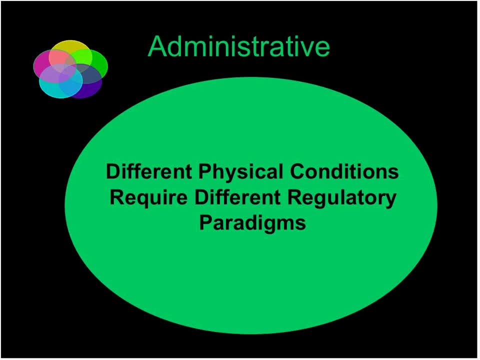 can be achieved and maintained for both the near term and the long term. The Nebraska system has a major advantage In that it recognizes the differences in both the physical conditions and other economic, social and environmental factors among different river basins and involves those most affected. 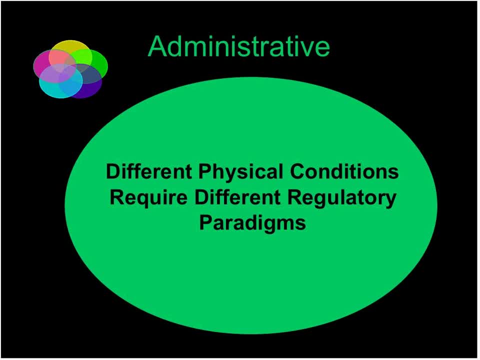 in the development of a management system most affected by the management system, in the development of the necessary rules and regulations needed to implement the management plan. But we must not forget individual basins are connected with each other. Therefore we need to enforce. 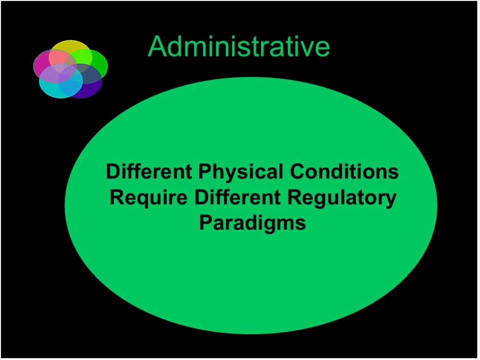 state-wide guidelines to ensure that what is done in one NRD basin does not adversely affect water use in another basin. The implementation of local control, either at the NRD level or a state level, has advantages, but it does exacerbate administrative problems. 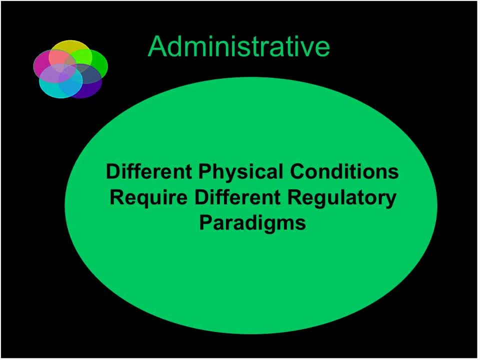 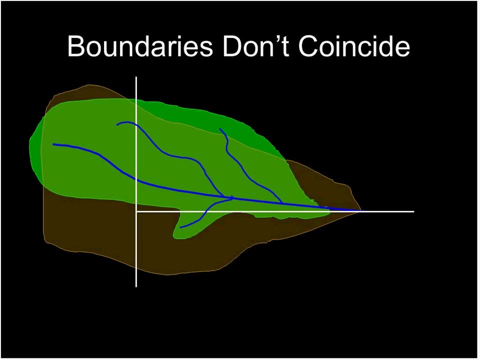 Water systems rarely respect jurisdictional boundaries. Often the impacts of a management decision are felt beyond the jurisdiction of the governmental entity or at the level of the management decision. This diagram shows the jurisdictional boundaries shown in white here, say of a state or a natural resources district. 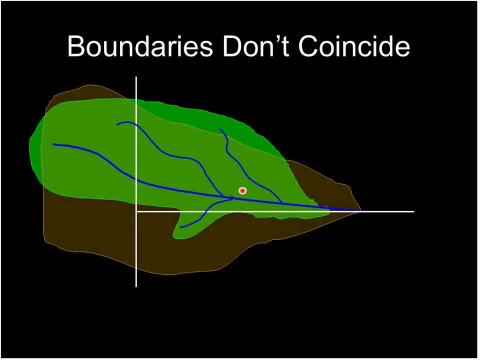 A stream is crossing. these boundaries, shown in blue and shown in green, is the surface watershed basin from which water runs off into the stream. The brown indicates the groundwater basin from which groundwater runs off into the stream. As you can see, none of these boundaries overlap each other or coincide. 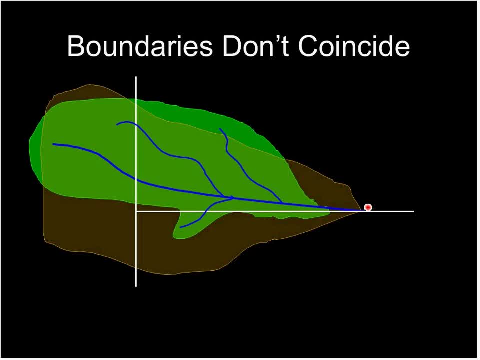 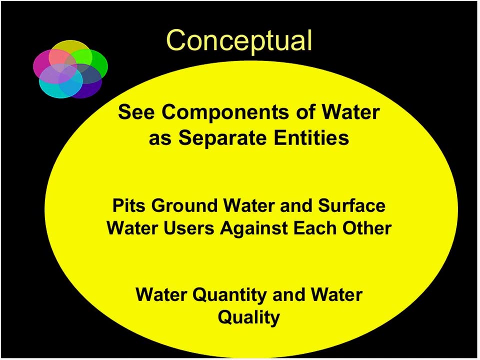 which creates jurisdictional problems that need to be taken into account as we manage more holistically both our surface water and our groundwater uses. In addition, there are a number of conceptual problems that I think we need to face, but, again, these also provide opportunities. 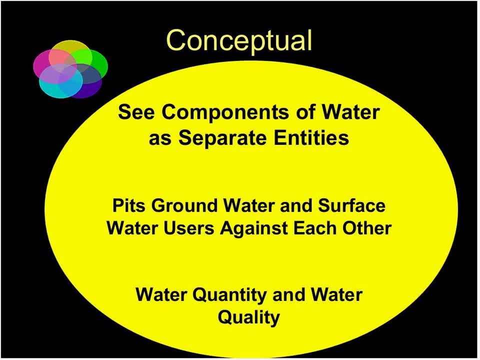 First, although we understand surface water and groundwater are hydrologically connected, we still view them as separate water supplies. This concept tends to pit surface water users and groundwater users against each other. In reality, where they are connected, surface water and groundwater are one resource and need to be managed as one resource. 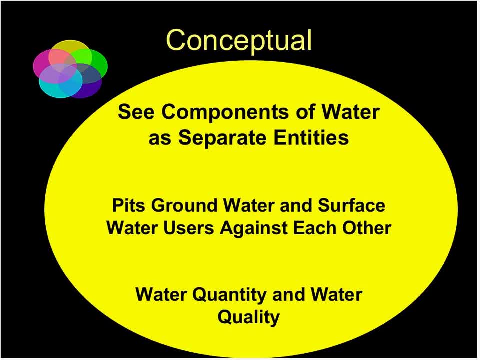 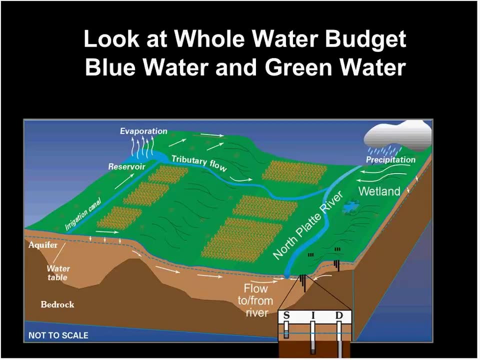 The exciting thing about Nebraska's new integrated management law is that it has the potential and in some basins already is fostering cooperation between surface water and groundwater users. Water quantity and water quality also need to be managed together. We also need to look at both blue water and green water. 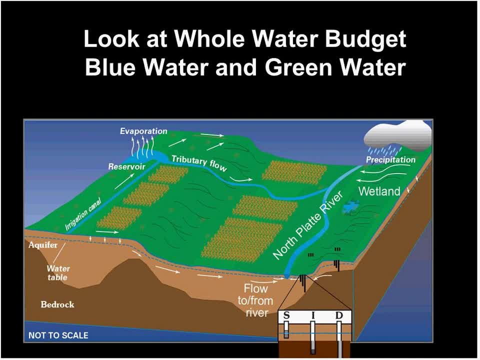 These are not separate water supplies, but are simply two different components of a single water supply and need to be managed together. What is meant by blue water and green water? According to the International Water Management Institute, blue water is the water in streams, lakes, groundwater, aquifers and in other words. 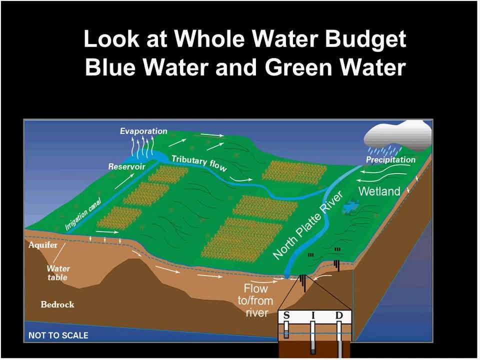 the flowing water that we usually think about managing, And green water is the water in the soil and land resources. Managing soil moisture through such practices as minimum tillage, together with the management of our streams and aquifers, I believe has the potential to enhance the beneficial use of all our available water supplies. 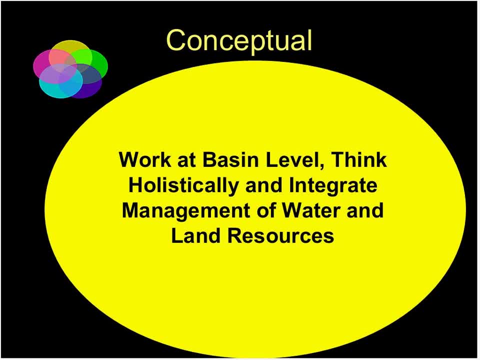 Thus, it is very important to ensure that the water supply is managed in a sustainable manner. It is also important to think at a holistic level and look at our basins as a whole. It is only in this way, I believe, that we will truly get a handle. 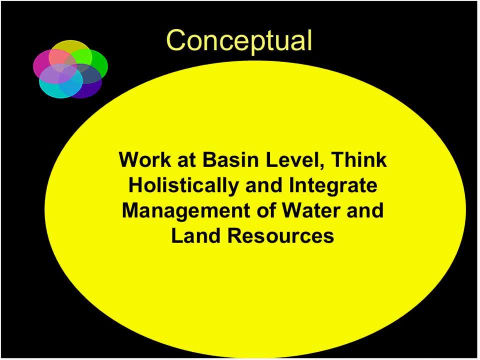 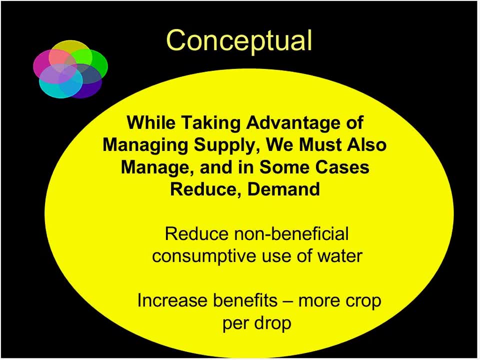 on our land and water resources. While taking advantage of water, managing our water supply, we also have to reduce our demand for water, And what this means is ideally reducing the non-beneficial consumption of evaporation of water while, at the same time, increasing the benefits we derive. 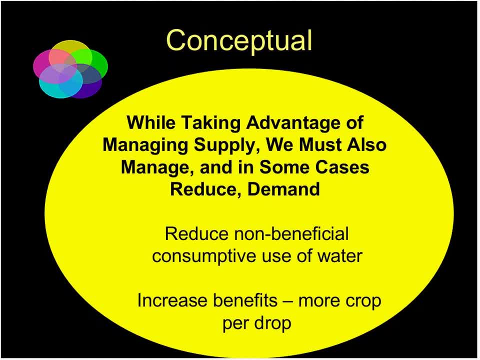 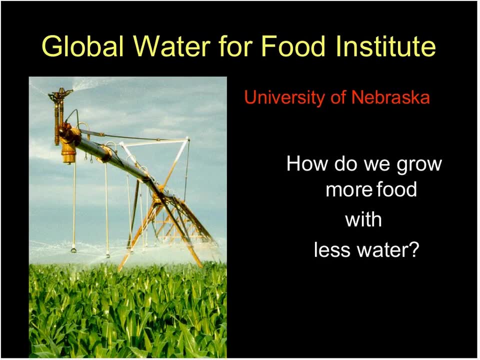 from whatever water is consumed. If we cannot do that, then obviously we will end up sooner or later as water supplies decline, reducing our overall productivity. But hopefully we will not have to get to that step To help answer the questions of how we can do a better job of managing our water supply. 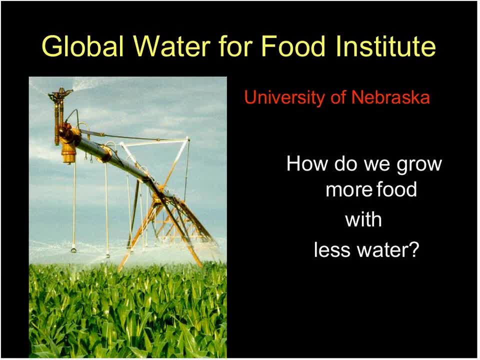 and actually produce more crop for drop, which has become the mantra. the University of Nebraska is establishing a global water for food institute. Hopefully this institute building on a lot of research that's already been done in the state with both water management and crop management and seed management. 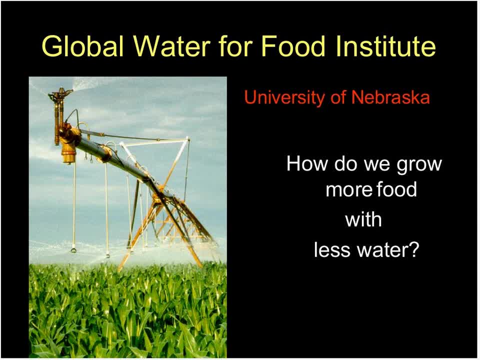 we will develop ways to grow more food with less water. The institute will focus on collaborating with natural and social scientists, engineers, policy makers and practitioners worldwide to make the knowledge of how to manage our limited water supplies for greater food production more accessible and help all countries to meet the global food challenges of the future. 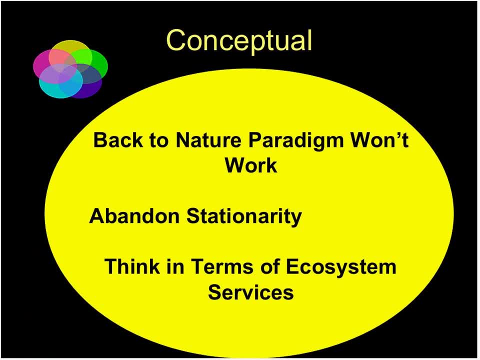 We also need to revise our thinking about the goals of water management. We should not set our overall goals. We should not set our overall goals as getting back to nature as we perceive it to have been in the 19th century or before. In my view, this will not work any better than the hippy back. 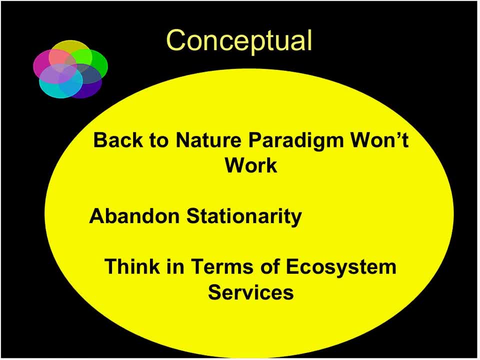 to nature farm movement did in the 1970s. We also need to abandon our assumption of stationarity, which is still used as the basis of many of our water supply analyses. This is the notion that it is the climate that will provide our water supplies of the future. 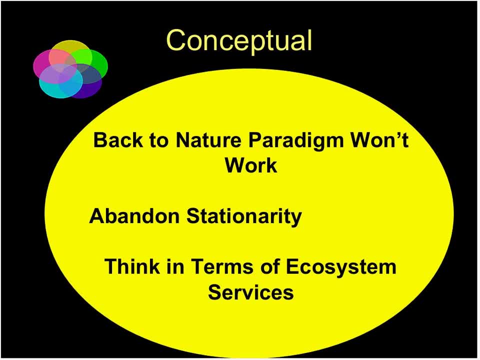 that the climate that will supply our water supplies of the future will be the same. It will be the same as the climate we've had in the recent past. Too often our modeling and management predictions are based on historical hydrographs of the last 100 years, yet the 20th century, in the US at least. 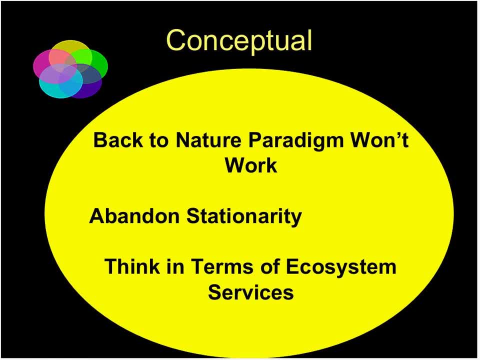 was one of the wettest centuries in the past 1,000 years. To think that these conditions will continue is foolhardy, especially given global warming. What we need to do is think in terms of ecosystem services, ie, analyze and make use. 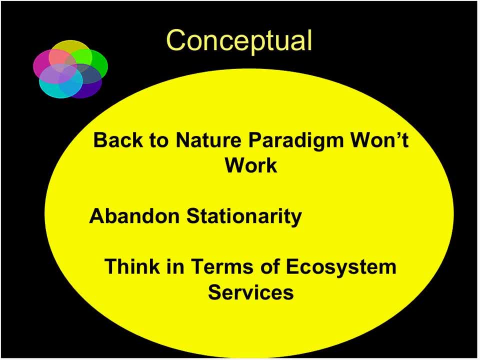 of the services that we have, The ecosystem has and could continue to provide, to enhance our quality of life. For example, we need to be mindful of the marshlands, that marshlands help manage floods and maintain high water quality. We need to look at our agricultural systems not as isolated fields but as part 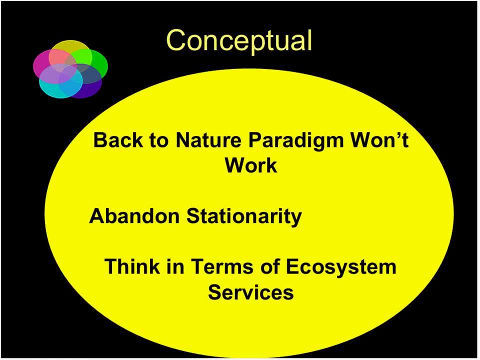 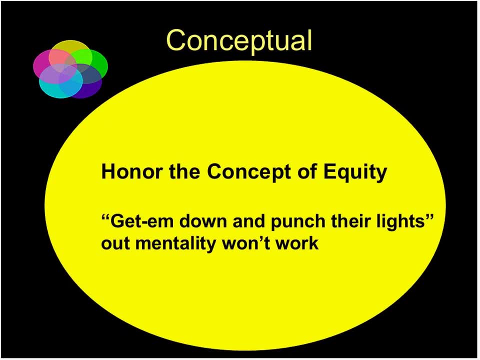 of a larger ecosystem complex which provides the basis upon which the quality of our life as a species depends. We also need to monitor the quality of our water. We need to monitor the concept of equity among stakeholders in the water basin. In my view, a get them down and punch their lights out mentality, while it may work, 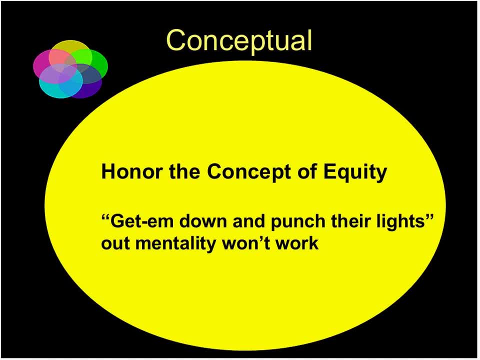 in the short run will not work over the long term, But treating stakeholders fairly and with respect can reap the long-term benefits that come from cooperation and collaborative decision making. In some cases it could, and already has, resulted in the ability to raise the funds necessary. 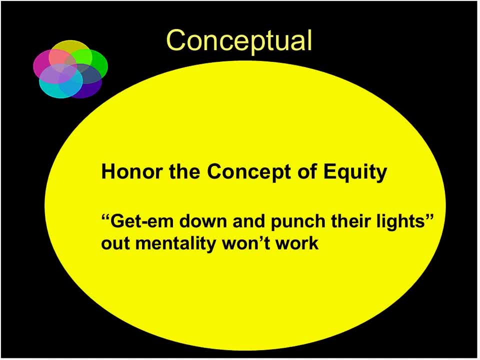 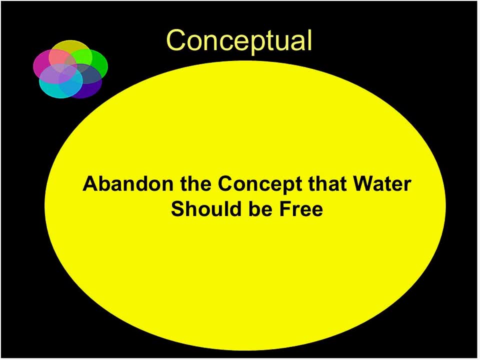 for good research and planning And to be able to buy out on a willing seller, willing buyer basis certain stakeholders when reductions in water use have to be made. We also need to abandon the concept that water should be free and treat water as a valuable commodity and recognize that value with mechanisms. 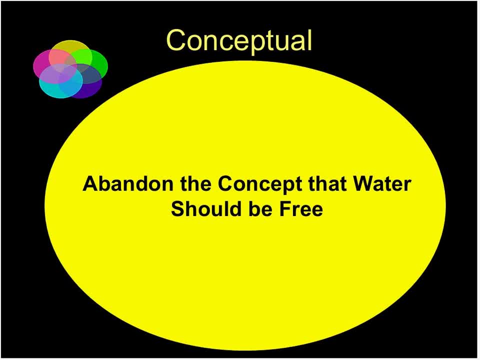 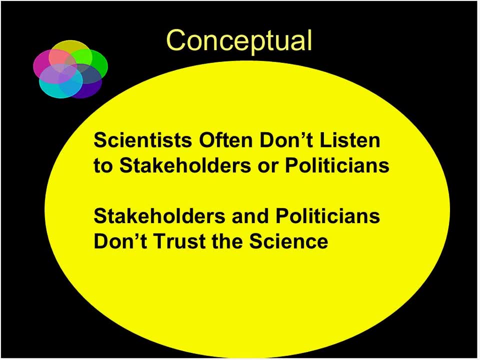 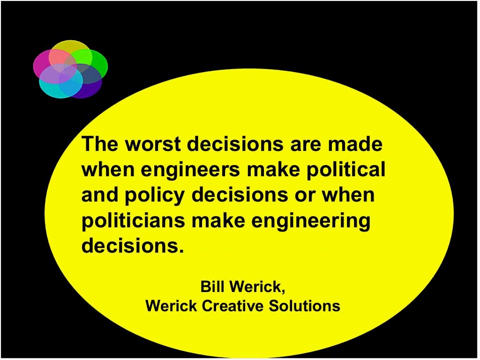 that price water at its true value. Another conceptual problem is that scientists often don't understand or listen well to politicians, and scientists And stakeholders and politicians don't understand or trust the science. The worst decisions are made when engineers make political and policy decisions or when politicians make engineering decisions. 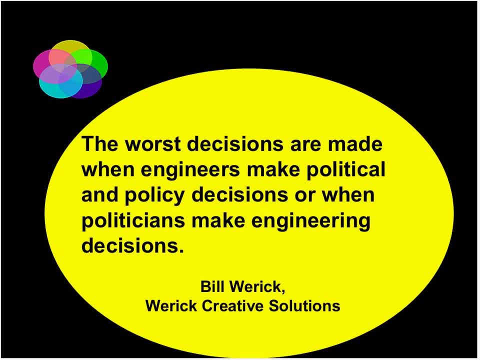 This is a statement made by Bill Wierick of Wierick Creative Solutions, while presenting the results of a study he has just recently completed. I'd like to share some of the results of this study with you, because Bill has been very helpful. Thank you. 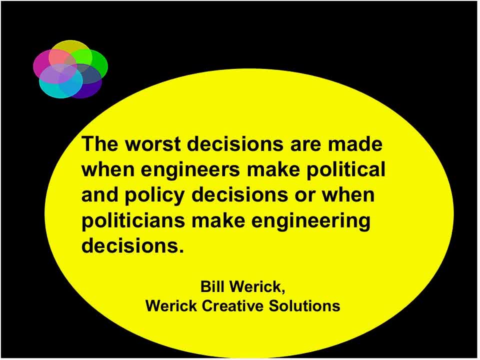 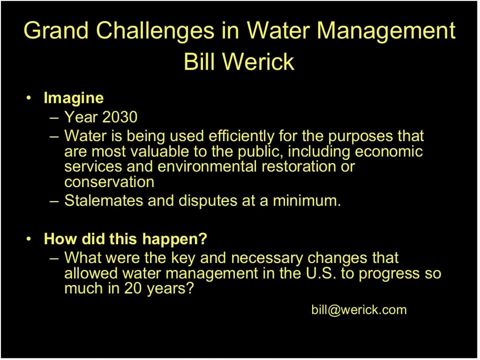 Bill's study suggests that there are more experienced and more smart people than I am who are thinking like me. In his study, Bill posed a question to a number of well-known international water planners and managers. He asked them to imagine that it's the year 2030 and imagine water is being managed. 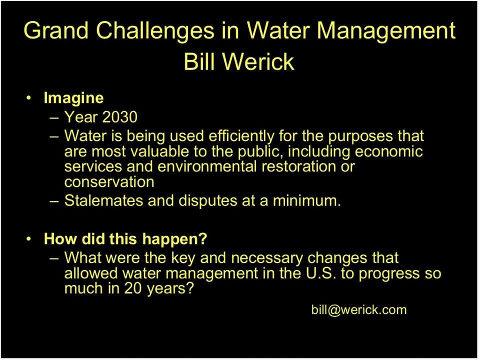 in the United States about as well as we can expect in a large, complicated democracy, He said. imagine that water is used efficiently for the purposes that are most valuable to the public, including economic services and environmental restoration and conservation. Imagine stalemates and disputes are at a minimum. 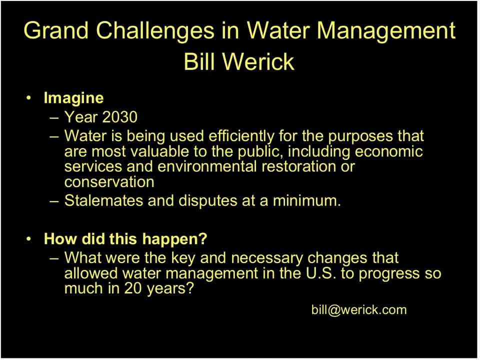 How did this happen? he asked What were the key and necessary changes that allowed water management in the US to progress so much in 20 years? A common theme mentioned by a large number of the people in the US is the importance of water management. 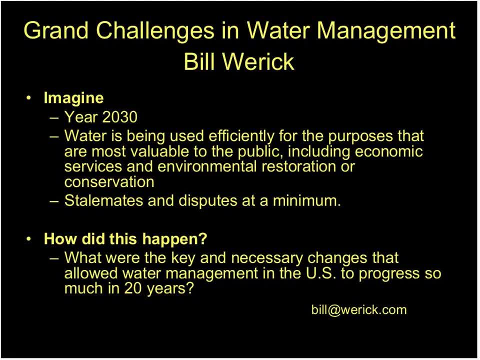 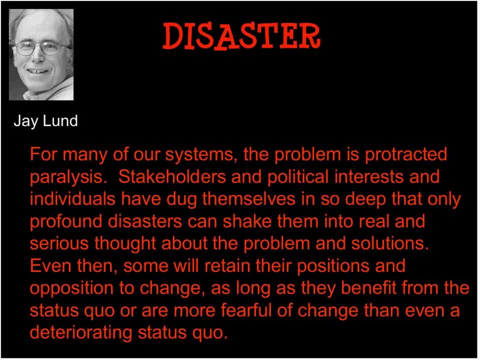 Bill's interview was well expressed by Jay Lund. He said we need a disaster. Lund said for many of our systems the problem is protracted paralysis, Stakeholders and political interests and individuals have dug themselves in so deep that only profound disasters can shape them into real. 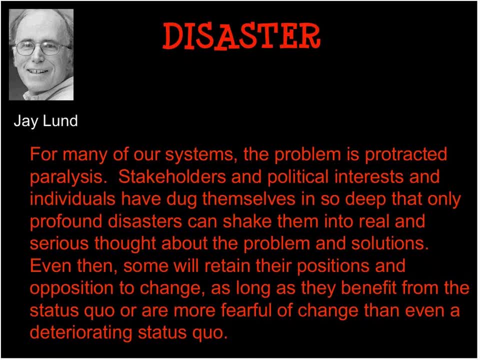 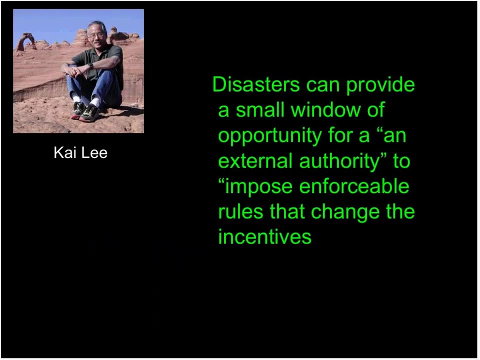 and serious thought about the problem and solutions. Even then, some will retain their positions in opposition to change as long as they benefit from the status quo or are more fearful of change than a deteriorating status quo. Kai Lee, a professor in civil engineering, echoed this in saying: 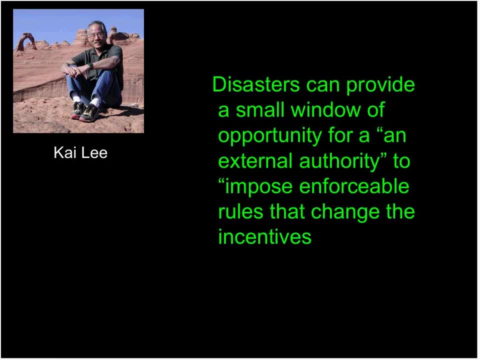 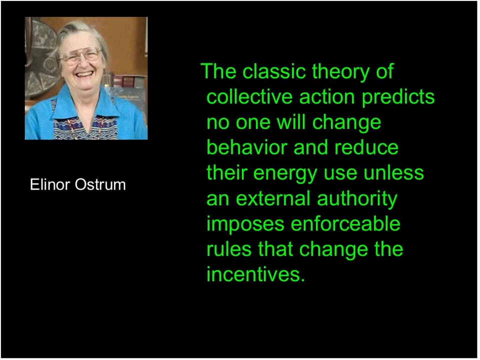 water scientists and engineers will not be the agents of change in water management, that such things are stubbornly resistant to change. however, disasters can provide a small window of opportunity For an external authority to impose enforceable rules that change the incentives. Thinking along the same lines, Nobel Prize winner in economics, Eleanor Ostrom, has said: 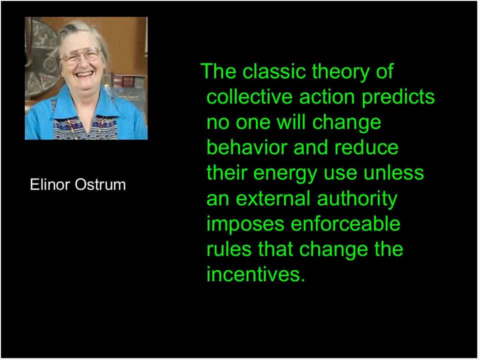 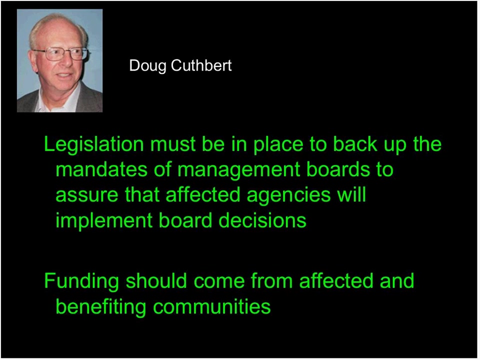 the classic theory of collective action predicts no one will change behavior and reduce their energy use unless an external authority imposes enforceable rules that change the incentives. She was obviously talking about energy use, but I believe the same concept. Doug Cuthbert, an engineer and scientist who's chaired many Canada-US water committees. 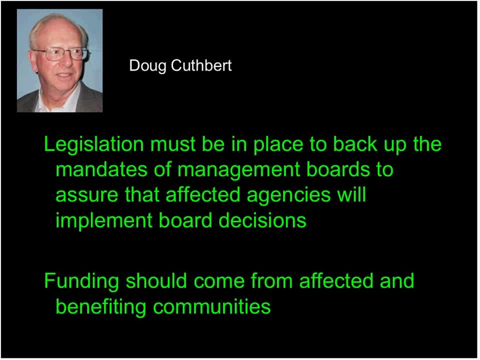 for the International Joint Commission said he definitely believed that there should be water management boards organized on a watershed and sub-watershed basis, charged with management responsibilities and decision processes relevant to their mandate and jurisdictions. These management boards can be regionally represented, politically accountable in general terms, but autonomous in that they would be empowered. 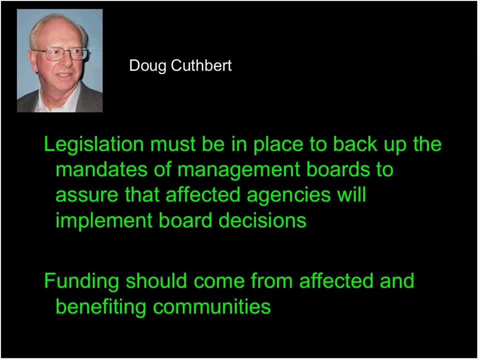 and mandated to make the best management decisions within specific deadlines. He also said legislation must be in place to back up the mandates of these management boards and to assure that the affected agencies would implement board decisions with funding provided from affected and benefiting communities. He concluded this is a challenge and a mouthful. 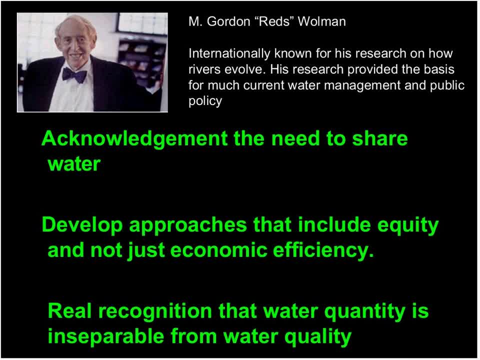 Gordon Reds-Woolman, who is internationally known for his research on how rivers and other surface water systems evolve and modify the landscape, responded that we need to acknowledge the need to share water and develop management approaches that include equity and not just economic efficiency. 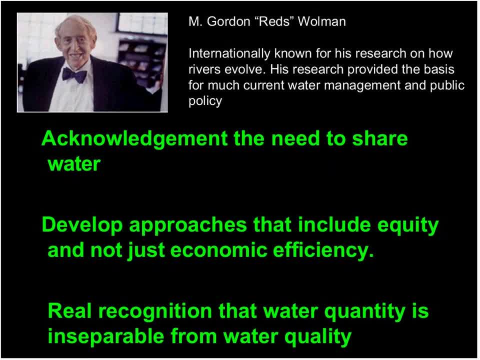 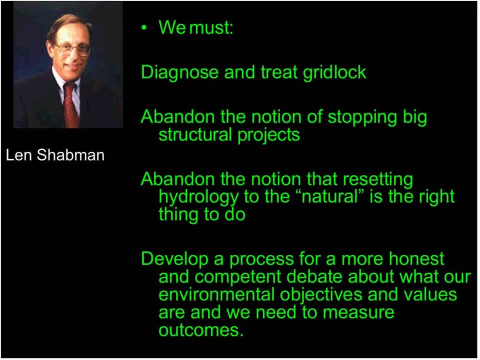 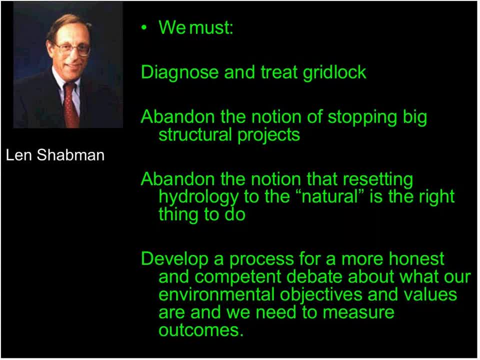 We must abandon the notion of stopping big structural projects and abandon the notion that resetting hydrology to the natural is the right thing to do. We must develop a process for a more honest and competent debate of what our environmental objectives and values are, and we need to measure outcomes. 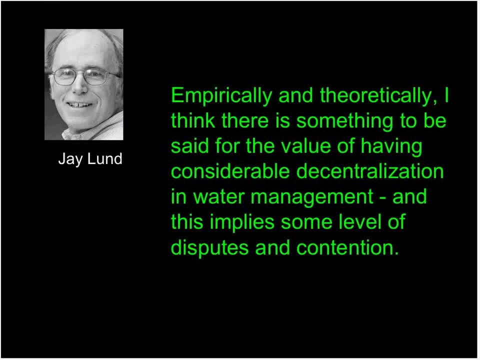 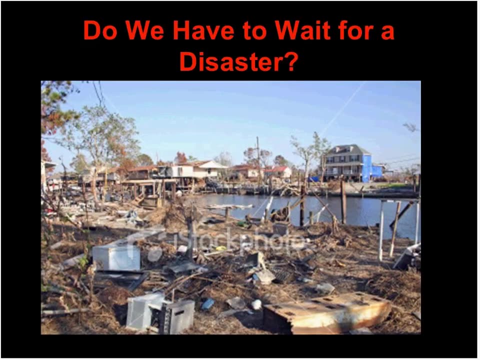 And finally, to go back to the question, back to Jay Lund. empirically and theoretically he said there is something to be said for the value of having considerable decentralization in water management, and this implies some level of disputes and contention. So do we have to have a disaster? 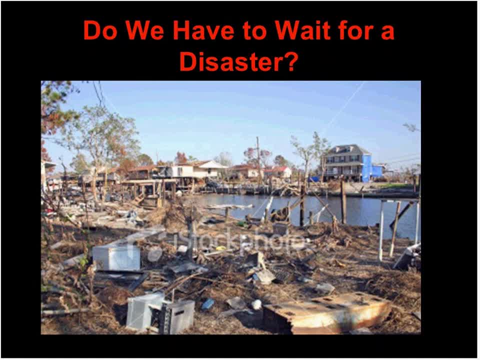 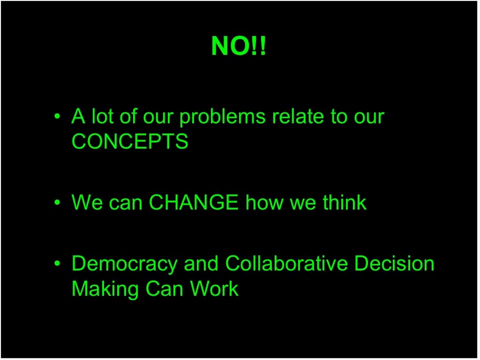 Do we have to wait or be like the boiled frog that sits in the water as it heats up without jumping out, sits there until he dies of overheating? I say emphatically no, because in part, a lot of our problems relate to our concepts or our mis-concepts. but these are challenges and these conceptions can be changed. 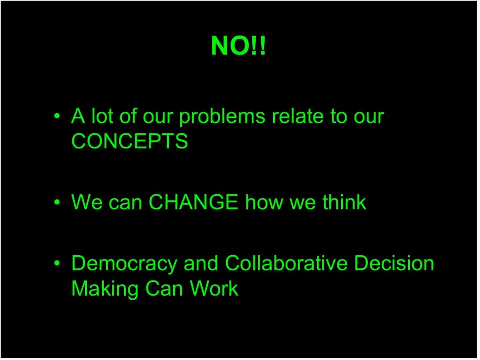 Science is providing some powerful tools for assessment and for developing ways to produce more crops or drops. but we need to be holistic in our thinking. We must not just focus on water, but look more holistically and include in our thinking considerations of the economic. 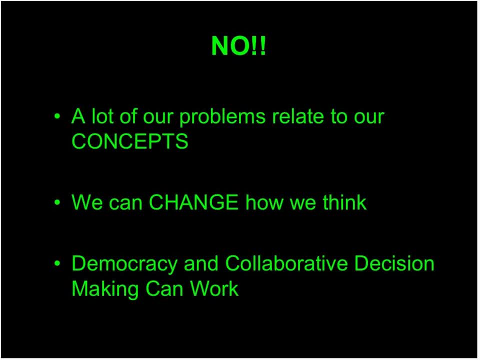 social and environmental systems that have such a large impact on the success of our management plans. We need to think not just about the individual unit, such as the irrigated field, but how that field fits into the entire ecosystem. We must be mindful of the overall health of our ecosystem services, on which we so critically depend. 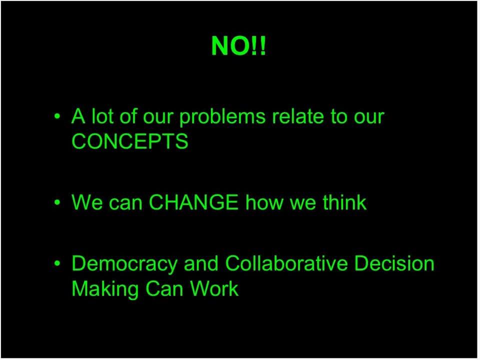 And although science, or scientists and engineers alone, or policy makers and politicians are not the only ones who are concerned, I do believe that the work of science and technology alone cannot get the job done. I do believe by working together with the affected stakeholders in collaborative decision making processes, we can succeed in meeting our challenges. 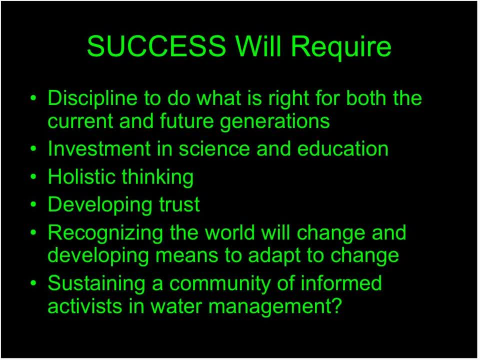 However, success will require discipline to do what is right for both the current and future generations. Investment in science and education, Holistic thinking, developing trust, recognizing the world will change- and development means that we have to adapt to that change- And, importantly, sustaining a community of informed activists in water management. 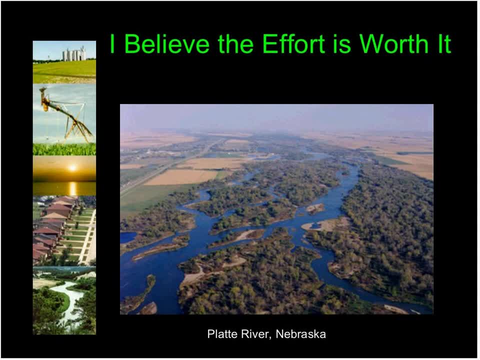 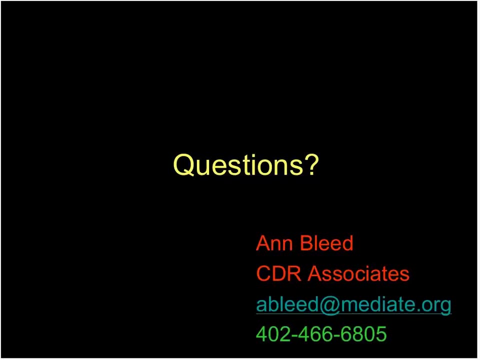 This effort will not be easy and will require significant sacrifice of our time and our economic resources, But when it comes to water, such a commitment, in my opinion, is both necessary and extremely worthwhile. Thank you for your time. If you have any questions, I will certainly try to answer them. 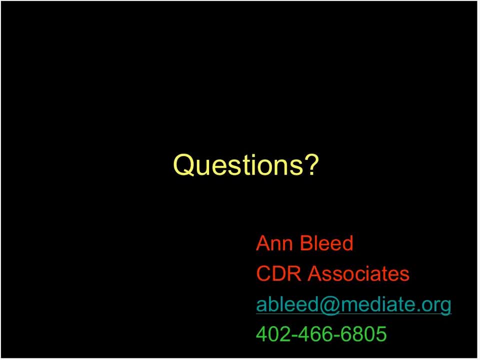 All right, Thank you, Ann. It is time for questions that we've received. If you have any other additional questions as we go along here, be sure to type them into the chat feature on the right-hand side of the screen. The first question I have, Ann, is how can we get stakeholders to think beyond their own need? 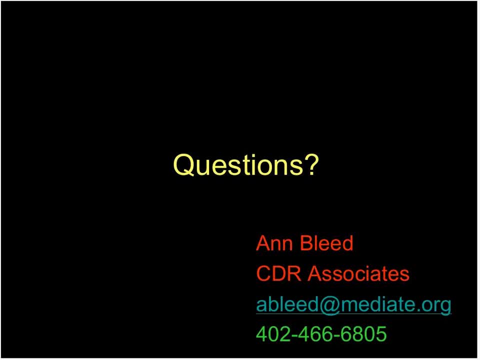 for the water and maybe what strategies can be used in that regard? That's an excellent question, and one that is always a challenge. My experience has been that, if you can get stakeholders together, both formally and informally, so that they start to talk with each other and start to develop a relationship, 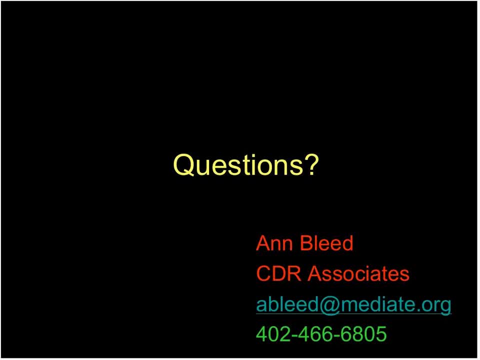 that you begin to see stakeholders starting to understand where the other stakeholder is coming from and starting to realize that these people have real concerns, And then you start looking for ways to satisfy, as much as you can, Other people's concerns as well as your own. 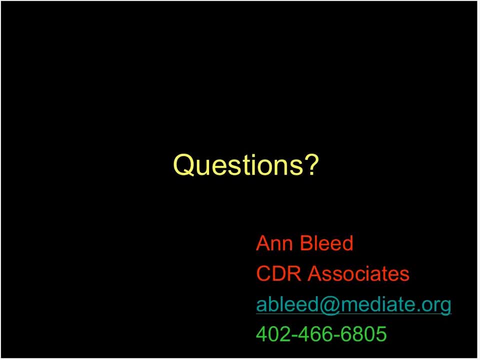 The other thing that I think it's important to do- and this is where science comes in: if you can look for alternatives that go beyond the normal way of thinking, that get us away from drawing lines in the sand, but start providing alternatives that might be solutions. 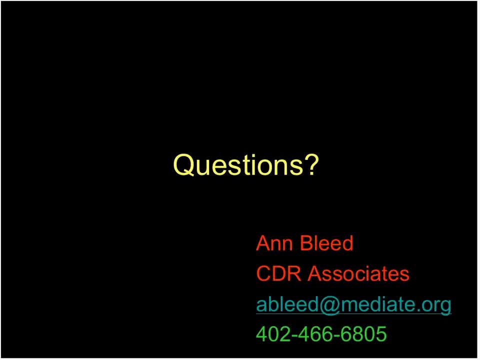 to more than one stakeholder's issues, that this can often help in bringing stakeholders together when they see a mucous, And I think that's one of the things that I think is important to do is to have a way to work together and to have a way to work together and to have a virtual benefit to working together. 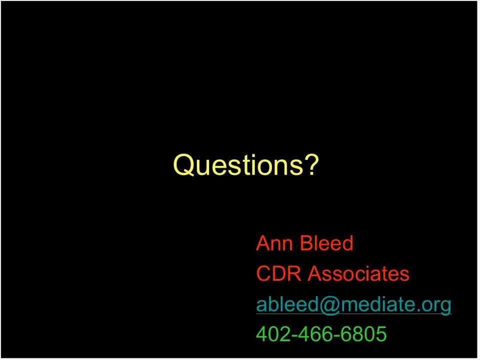 Another question- maybe seems like maybe a little on those lines- is: do you think we need some sort of level of water management on a federal level, or a body that can look at the resource as a whole in that way? Well, that's something that has been debated, as many water policymakers know, for many. 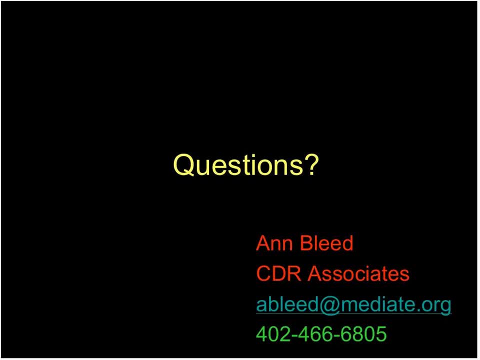 many years, and going back 30 years or so, we did have water basin commissions that were organized. I think in some ways. yes, my comment about making sure that we have rules in place that ensure that local basin management decisions do not adversely affect other basins is critical. 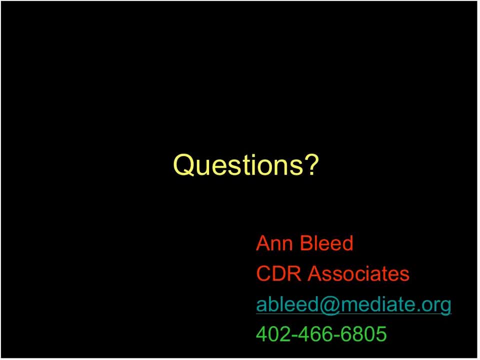 and we also need to make sure that the enforcement guidelines are in place to make sure that the local entities that are managing water do in fact, do what they need to do. However, I do think that we're better off working at a local level as much as we can on water issues. 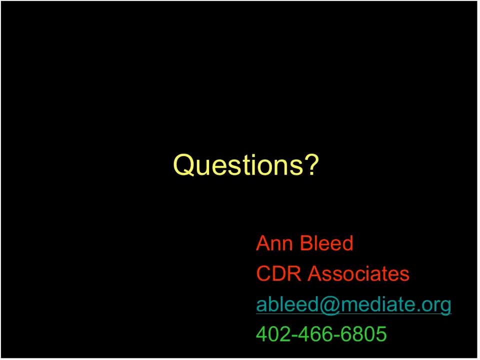 because our basins throughout the United States are so very different and actually the values that people bring to water use in those basins can be very different from one place to another. So I think local control, but with some kind of overarching guidelines that can and will be enforced if necessary. 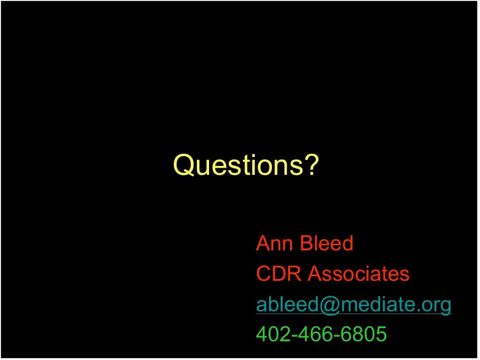 To make sure that those at the local management level are fulfilling their responsibilities. Okay, So how do you feel? how you measure the success of integrated water management? I think the success of what we do today will really be measured 20,, 30,, 40,, 50 years from now. 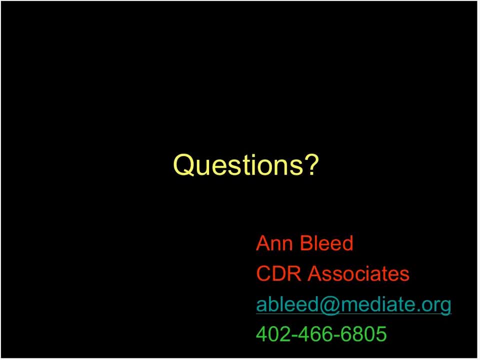 That's, unfortunately, one of the difficulties that I've had to deal with. I see, on a current day basis, I think the lack of disputes would be one indication that we are successful in what we're doing and to the extent that we do have litigation and conflict, 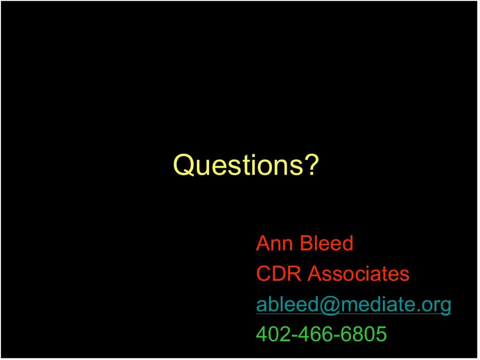 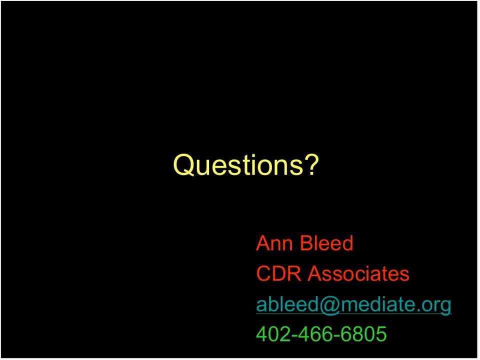 Okay, Right now, no, Most people are not charged for the use of natural flow, And that's what I meant by the need to recognize the economic value of water. The problem we've got is, although we pay for infrastructure to get the and move the water, 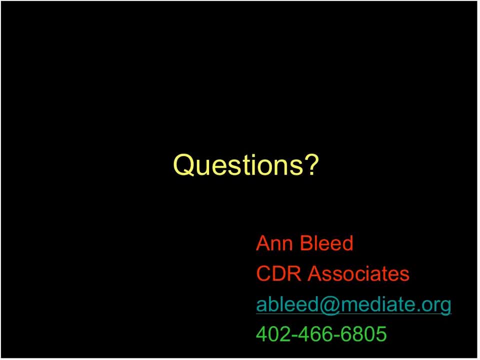 and pump the water from one place to another, we are usually not charged for the water itself. We tend to take it as a given, And so, Therefore, I believe we do not respect it as we need to respect it. There is a value, in my view, to natural flow in streams. 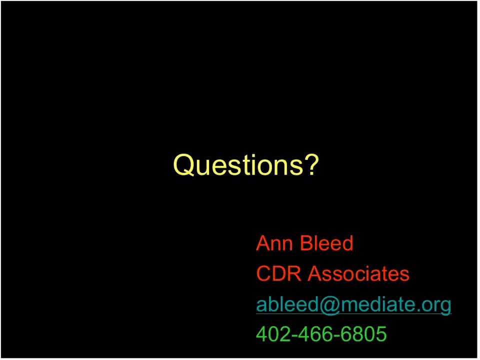 And this is where I think we need to look very carefully at what our values are on a basin-by-basin basis, And if, in fact, we do value having natural flow in the stream, either for fish and wildlife purposes, or for recharge purposes or water quality purposes. 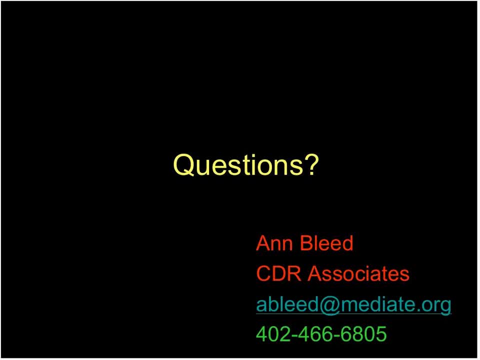 I know in Nebraska there are a lot of cities that depend on stream recharge for their municipal drinking water supplies. Where those values are clearly articulated and recognized in a management plan, I think we will start to put a value on in-stream flows And I think eventually we will have to put an economic value on that water. 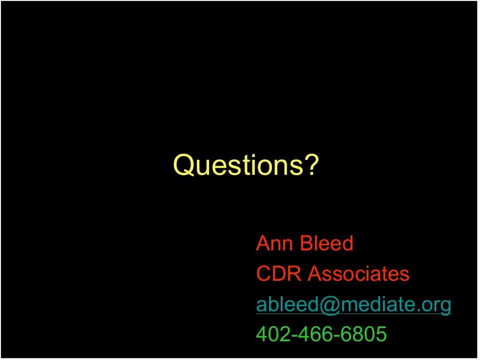 and that water will be used for drinking water And so that we pay the appropriate price to maintain it. Another question: how does population growth rate affect how we manage water? Well, clearly, population growth rate increases the demand for water and makes our job much more difficult. 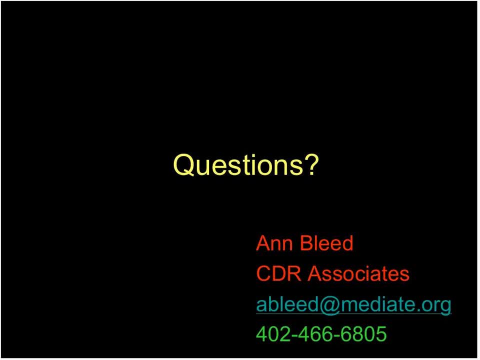 At a conference where we looked at the Global Water for Food Institute and how it should be set up. it was commonly said that in order to meet the world's population demand for food in 2050, we would have to worldwide double our food productivity, which is one of the motivations. 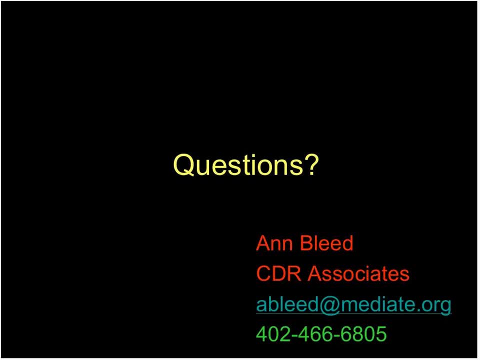 for the Global Water for Food Institute, But that also creates tremendous demand on our water supplies, and I think that we're going to see more and more emphasis placed on water, not only for drinking water, but for the production of food. In the process of doing that, however, I think we need to be very cognizant of the fact. 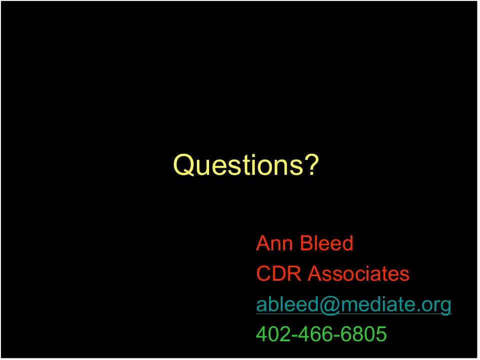 that we cannot destroy the ecosystem on which our society depends and we have to be mindful of those other ecosystem services. That's not to say we have to go back to what the ecosystem looked like 100 years ago, but we do need to be mindful of the ecosystem. 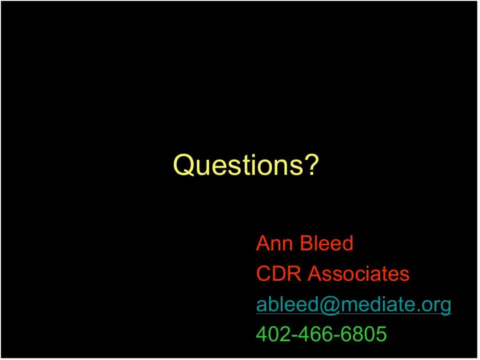 And I think that's something that we need to continue to do as we move forward with the services those ecosystems are providing and hopefully will continue to provide for us as a human species. Another question is: what's a good resource for a lay person to get a really good explanation? 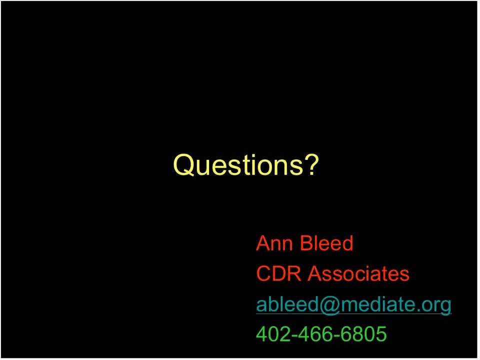 of Nebraska's water law. There are some publications that came out of the Department of Natural Resources, some pamphlets that do a brief job of describing the resources that are being provided to us, And you can find that in the National Water Agency website. 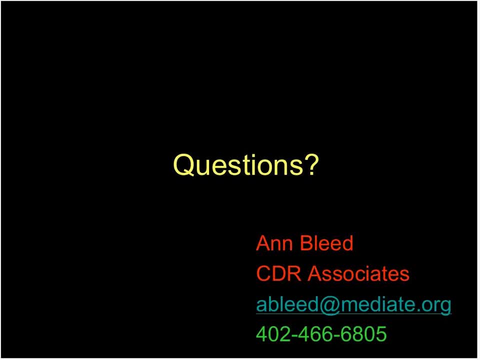 You can find that there are several resources that are available to you. job of describing Nebraska's water law. Beyond that, I don't know that anything has been actually written down And, as I said, the new integrated resources management law is still in its experimental stage and time will tell whether it works or not. 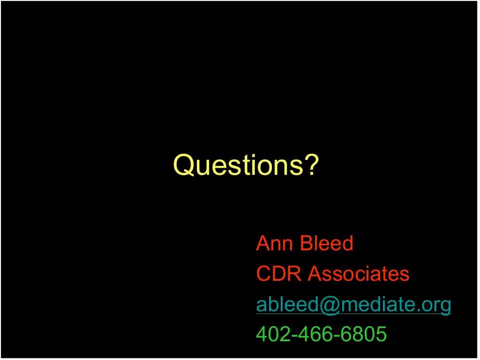 A couple of questions in regards to Australia, And I mean one of them maybe, is what are some lessons that can be taken from that plan that they have? Well, I am not an expert on Australian water law by any means, But I think there are a. 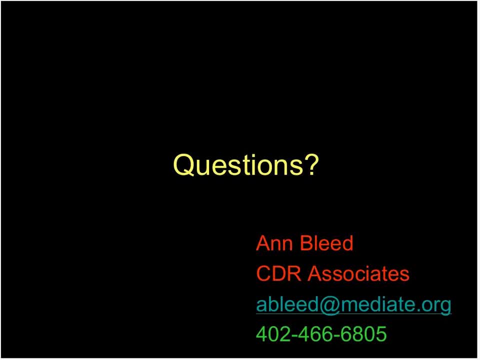 couple of lessons. One is that, and perhaps a very important one, in Australia they truly believe that climate change is a reality And, instead of assuming that the water supplies will continue in the future as they have in the past, they have really come out with a 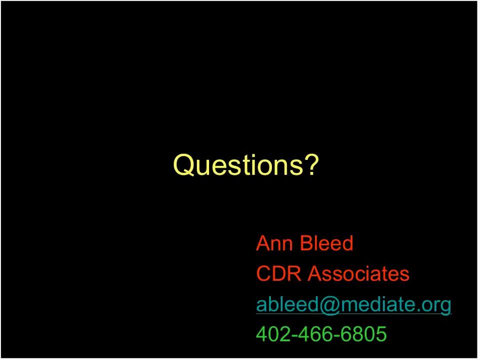 grip with the fact that they have a change in their climate which is very adversely affecting their water supply. They have also been very active in trying to work together to reduce demand. I know that most households in Australia have been given an egg timer of four minutes. 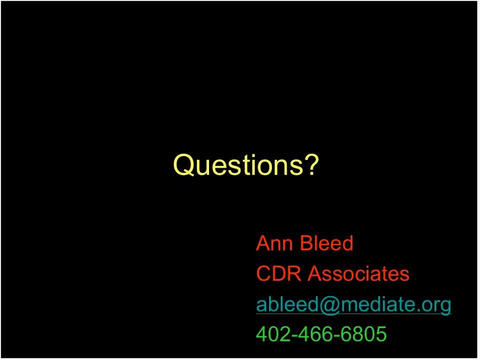 And the goal is to make sure that your shower lasts no more than four minutes And they feel that they have a better chance of staying dry in Australia than if they were not. The other thing that has happened on the children's program: there are songs that children are. 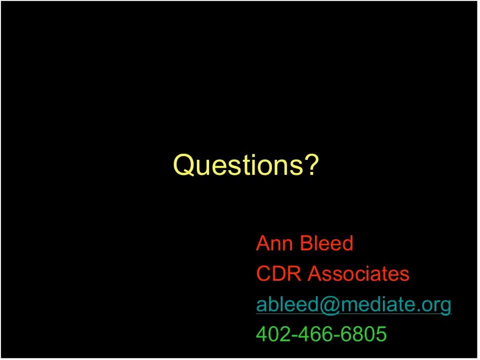 singing at great lengths- And I know this because my grandchildren live in Australia- saying: don't waste the water, it's precious. In terms of actual changes, they have been evolving. it hasn't been a massive all of a sudden change, But they have been involving their water law system so that they don't. 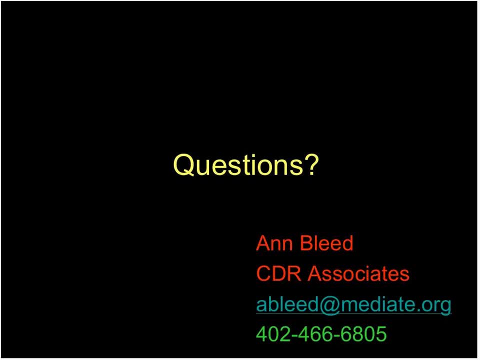 look at the rates of diversion as much as the total. This has been important And I think, as you all said, that has been an important piece of the program for us- And what has as the total quantity of diversion and they limit how much both surface water. 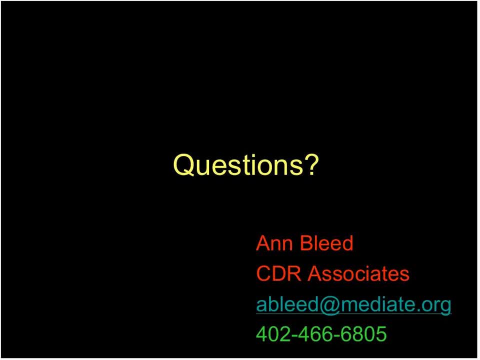 and groundwater can divert for a given use in terms of quantity per year, and this is happening to some extent in Nebraska with our groundwater resources and I think it will continue to move across the state and perhaps be expanded to the use of surface water, where you would have an actual biometric. 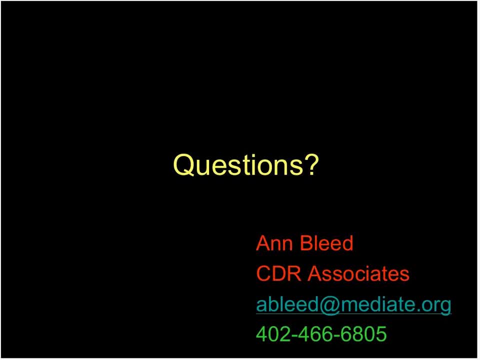 amount within which you must with. that is limiting your use and therefore you must make do with and expand your productivity given that limited volume. but there's a lot more to Australian water laws, and then I know that I'd like to learn more. I think we have quite a few engineers joining us today, and one 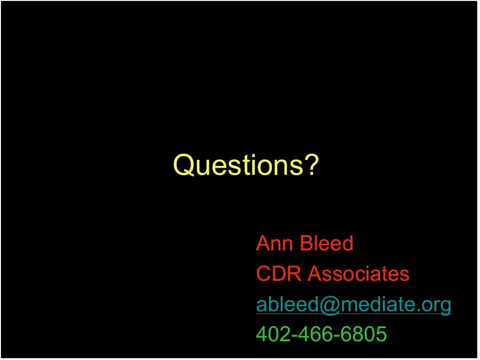 of the one of the questions that's asked is that that you mentioned. one of the problems is that engineers are not as good as they should be, as engineers are not as good as they should be. engineers are not as good as they should be, as engineers are not as good as they should be. 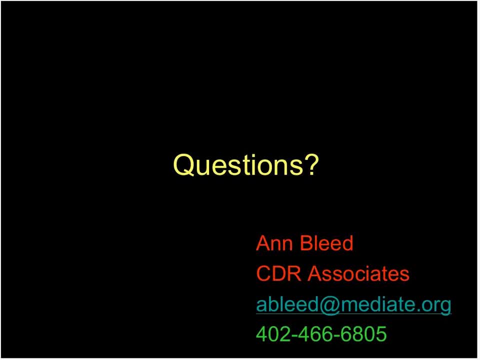 Engineers try to make policy decisions and politicians tend to make engineering decisions, And the question is: as engineers, it would be great to hear what are some common examples of policy decisions that engineers tend to make that maybe they shouldn't. Is there something you can think of? 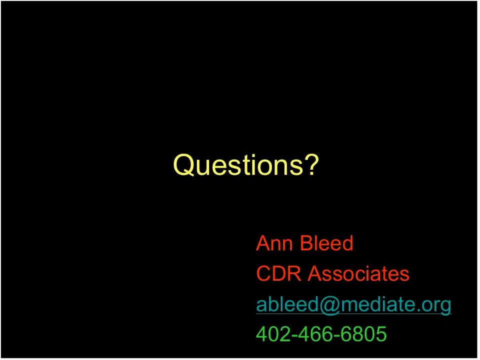 Well, what I have seen is situations where engineers will develop a model for a system and come up with what they believe is the right solution And present this as the solution, And when this type of thing does happen, I think that it tends to be a fairly narrow solution. 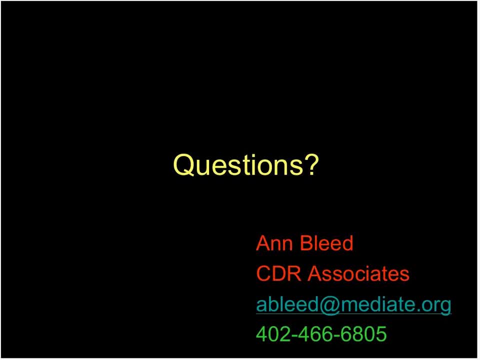 and often omit something that might be very, very important to stakeholders, to the point where the stakeholders say no, we will not accept this, And of course then the dispute only increases in volume and nothing gets done. But I really do believe by working. 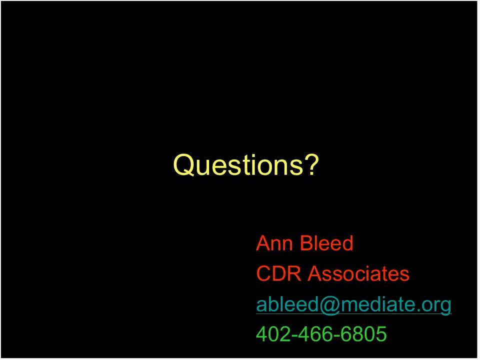 together, the engineers and policy makers can really come up with a superior solution that recognizes things beyond the pure engineering principles, that recognizes the social and economic and value systems of stakeholders. Another question: does integrated management include recycled water supply? I think it certainly can. 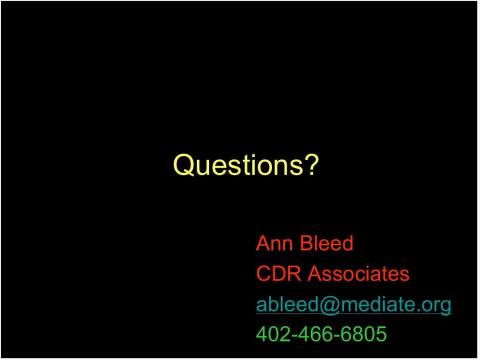 And in terms of water supply, I think it certainly can And, in fact, I would argue, probably it does, necessarily because we deal with a hydrologic cycle, And I do think that one way that we can expand our efficiency of water use is to recycle water. 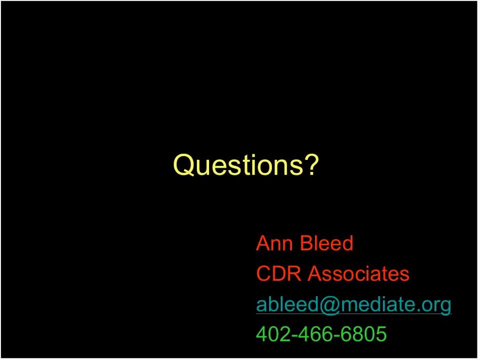 When I mentioned the incidental recharge of ground water aquifers by the diversion of surface water for irrigation. that is a recycling of water And in Nebraska we have a lot of water recycling And in Nebraska on the North Platte River that kind of a system which was started in the 1900s. 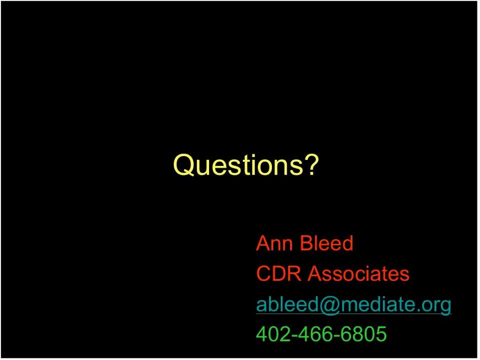 when we started diverting water for Bureau of Reclamation lands created a tremendous recycling system that has proved to be very efficient all the way down to two-thirds of the way across the state. This is not the intention of the early planners, but that's in fact what happened. 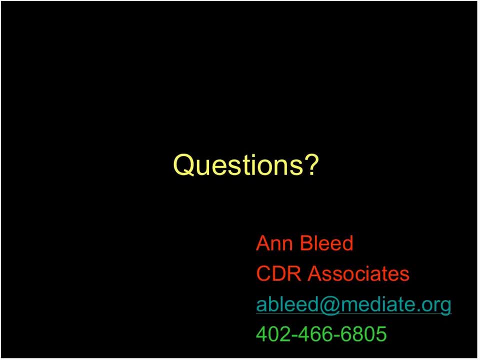 And I believe that if we focus on that more carefully, as is being done in Nebraska and Idaho- and I know a number of other states- that we can make more efficient use of our water through recycling. I think the final question today is- I think it kind of bodes into the future then. 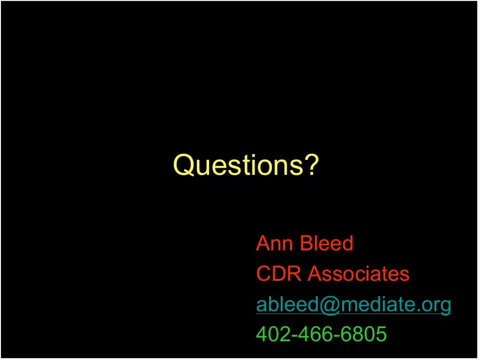 is, if our measure of success is to be found years in the future, how do we motivate change towards success today and into the near future? Boy, that's a very good question and one that I've struggled with a great deal. Thank you. 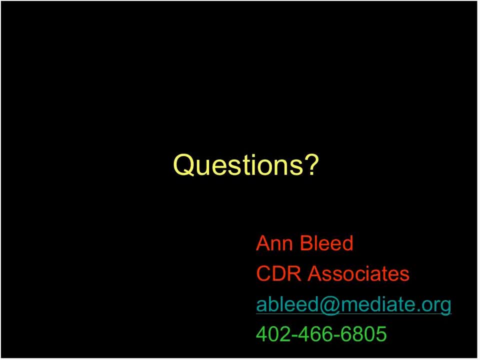 Trying to survive. the economic times of today is critical, especially to farmers and farming, and agriculture provides 90% of the consumptive use of the water throughout the world. Farmers are struggling just to survive the next year or the next few years, and to ask them. 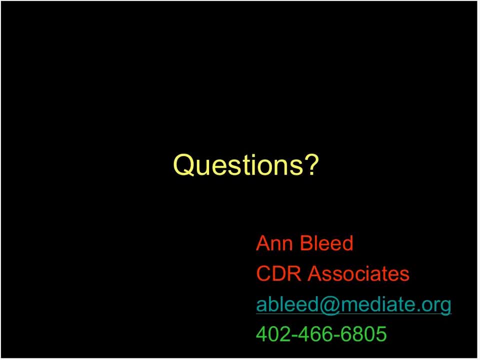 to think about restricting their water use so that somebody can have it 30 years down. the road is really really tough. On the other hand, when I think you, when you talk to folks, you find out that they are concerned about what kind of a world we'll have for our children and grandchildren. 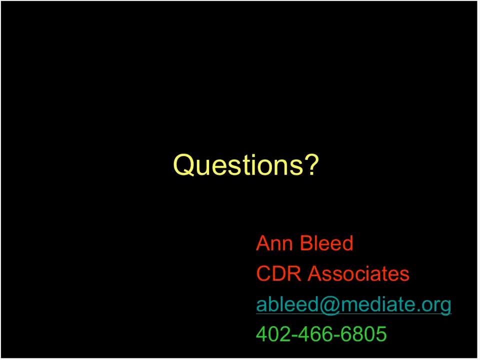 So I think one of the ways that I see success is trying to get a better handle on what our consumption of water is in a basin and what kind of water supplies we have in the basin, and bringing those into balance in both the short term and the long term. 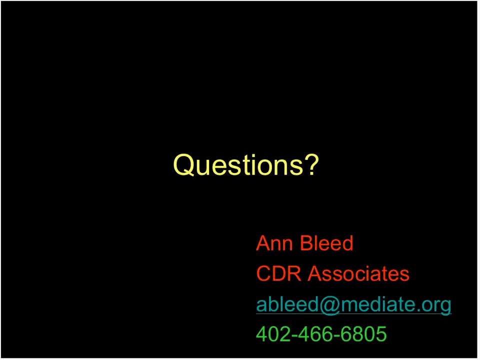 That doesn't mean in a dry year you can't use a bit more water from the aquifers than you otherwise may would in wet years, with the understanding that those aquifers will recharge. but over the long term I think that if we can come into a balance between our supply and use, we'll be in very good shape for the future. 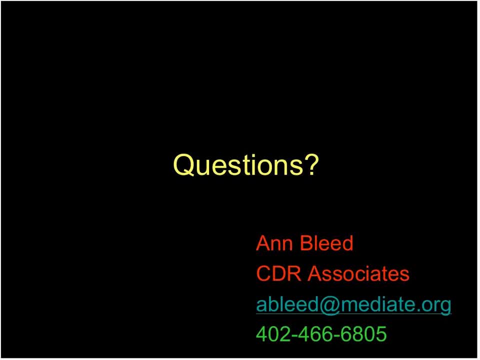 And that's again where science and modeling comes in, because we have to try to predict what that balance is and what it will be in the future. but there again I think we are. we're developing better and better tools to make those predictions and as long as we don't rely 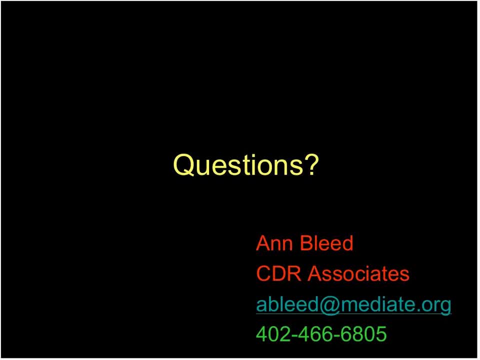 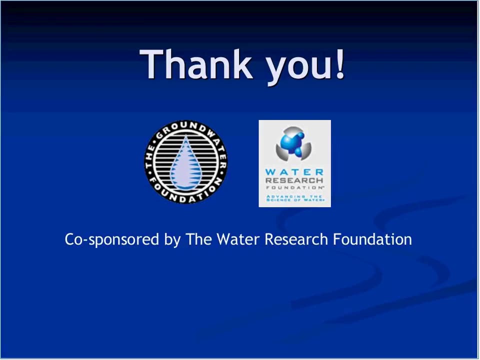 on the stationarity of climate change. I think we have a reasonable chance of using those tools to come into balance and use that actual balance as a measure of our success. Great Well, I just want to say thanks again for to Ann and for everyone. 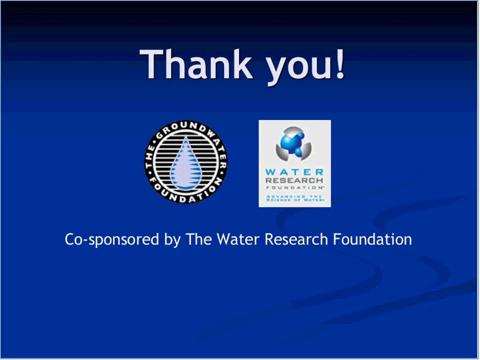 for attending today's webinar that's co-sponsored by the Water Research Foundation. After today's webinar, we'll be back with another webinar. You'll receive a survey evaluation for this and via email from us, and if you have a chance to fill that out and respond to that, that'd be great. 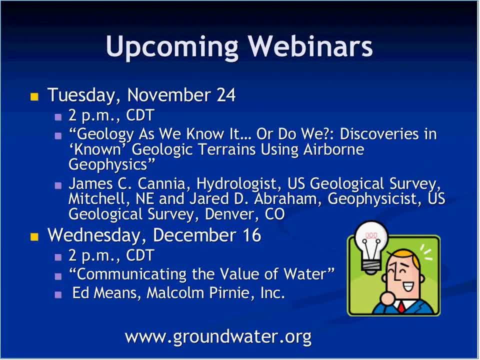 Our upcoming webinars. the next one is on Tuesday, November 24th, where we'll discuss geology as we know it, or do we discoveries in known geologic terrains using the airborne geophysics. The registration for that will open in early November at our website.